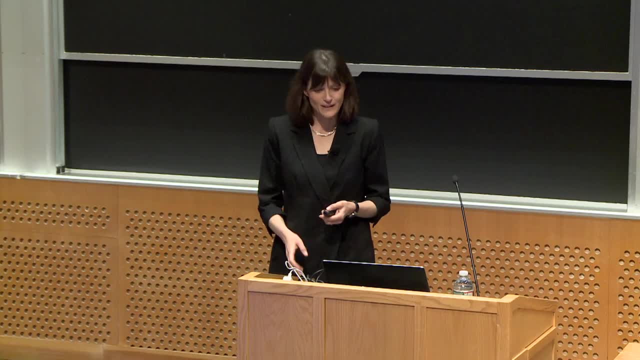 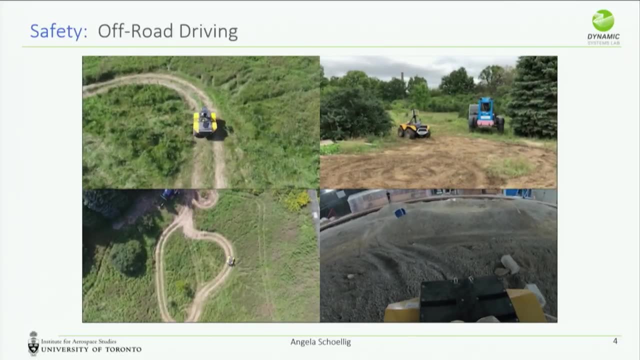 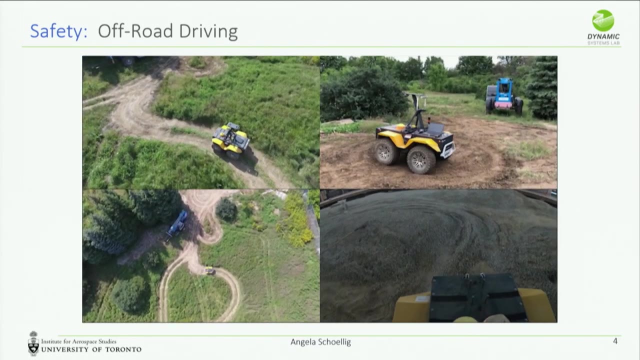 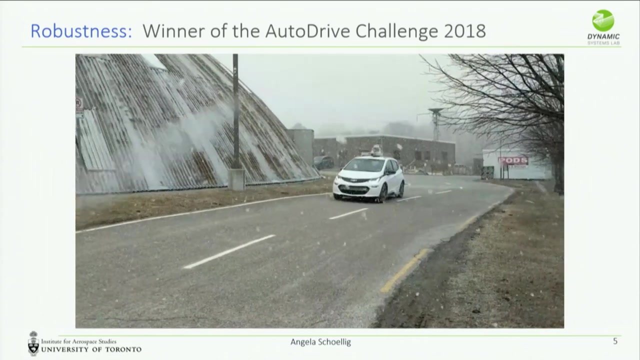 And so we want to fly these vehicles reliably, given that they're outdoors and quite heavy and dangerous, Also drive outdoors in varied off-road terrain, And safety here means that we don't get off the path while trying to optimize the performance and the speed of this robot. And finally, we are part of a self-driving car competition. 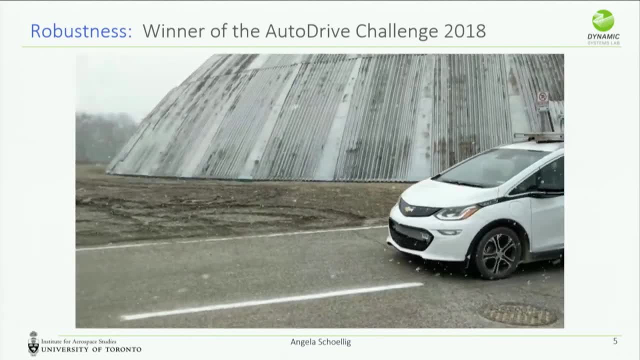 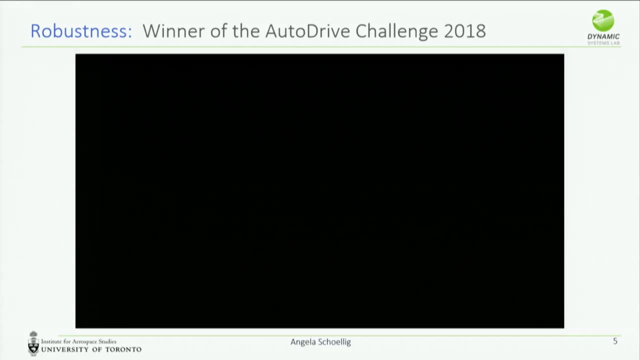 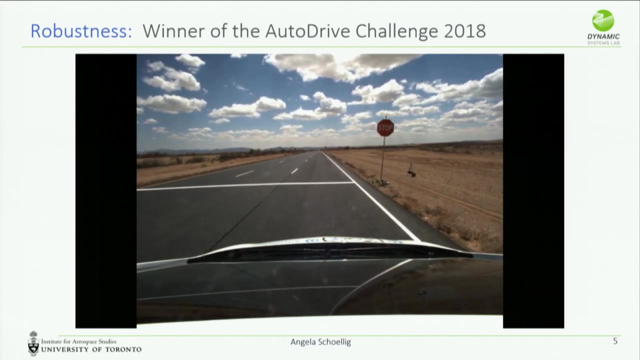 and we had to test in winter conditions in Toronto And our algorithms, our algorithms had to be robust enough to drive at the competition in the desert in Arizona and we had exactly ten minutes to tune any of these algorithms. So what all these examples have in common is that these robots must. 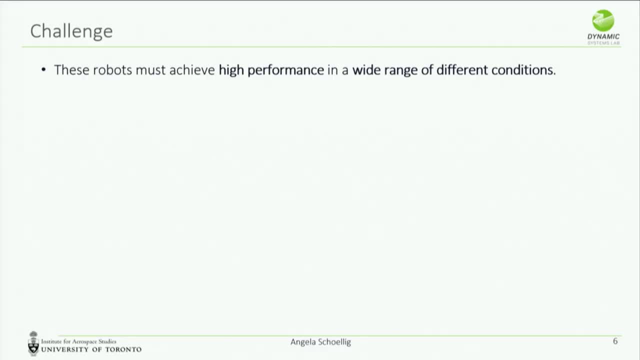 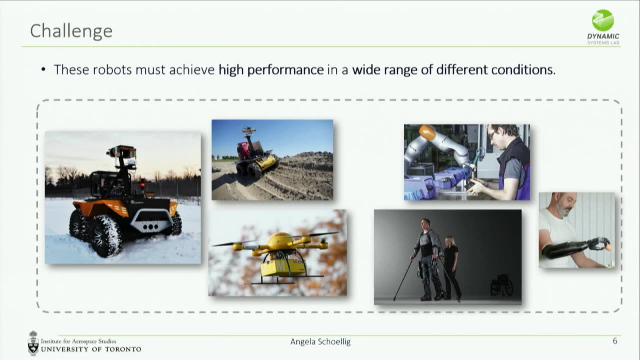 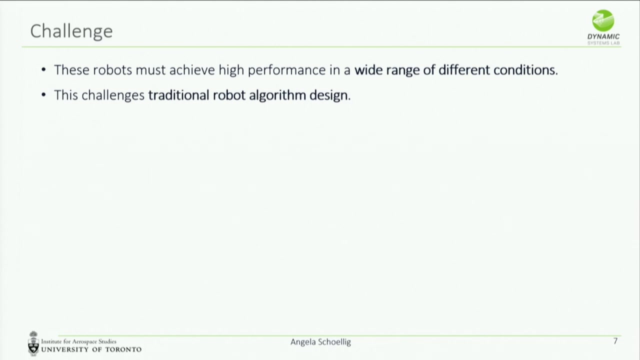 achieve high performance in a wide range of different conditions, And these conditions can be environment conditions, but in the future, different conditions may mean working with different people And in collaboration- collaboration with people- And this generally challenges traditional robot algorithm design, which looks usually like this. It's kind of a closed loop. obviously We have sensors. 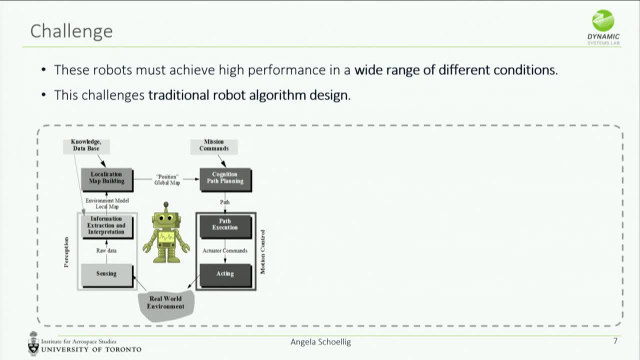 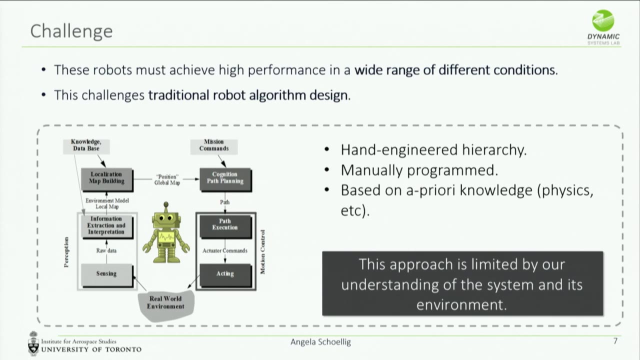 then some state estimation, mapping, a planning component and eventually motion control. And all of this is hand-engineered, It's manually programmed and based on a priori knowledge, for example first principles models of the robot. So this approach is limited by our 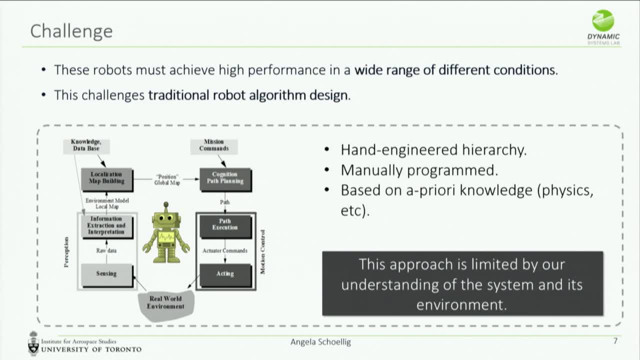 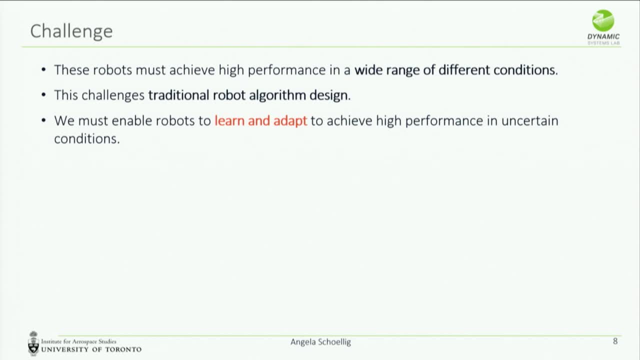 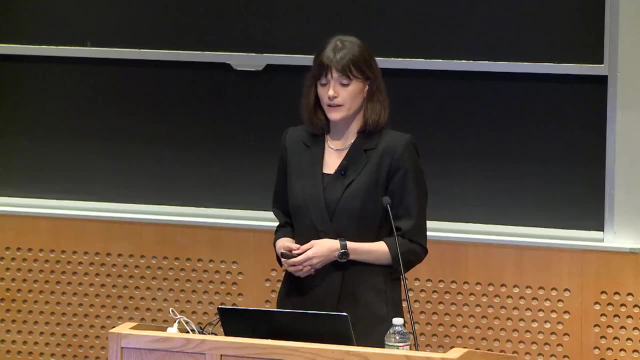 understanding of the system and its environment And to enable the applications I showed you in the initial videos, where we have a wide range of different conditions. we really have to enable robots to learn and adapt to achieve high performance in those conditions. So learning 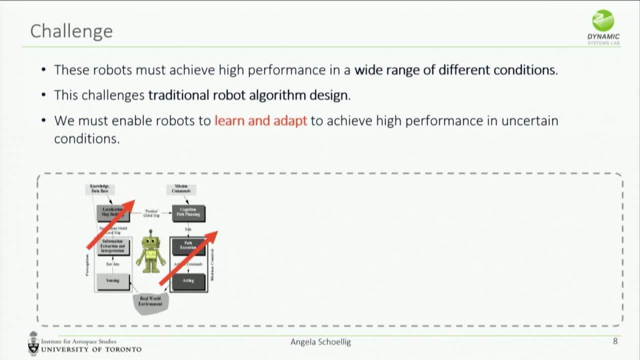 and adaptation in this case can mean many, many different things. You can put a learning component in every module, in your vision module, in your planning module, in your control module. You could do VOM, big neural network, end-to-end, from pixels to volts. So I think one really big and interesting. 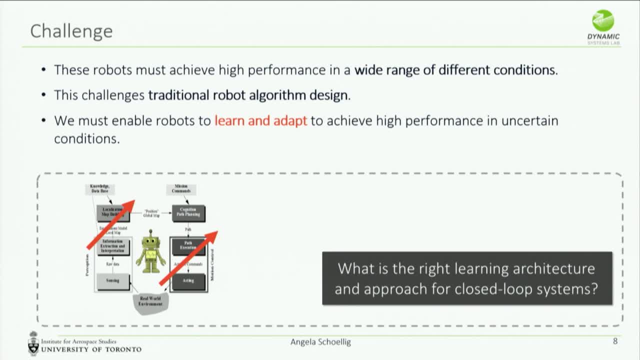 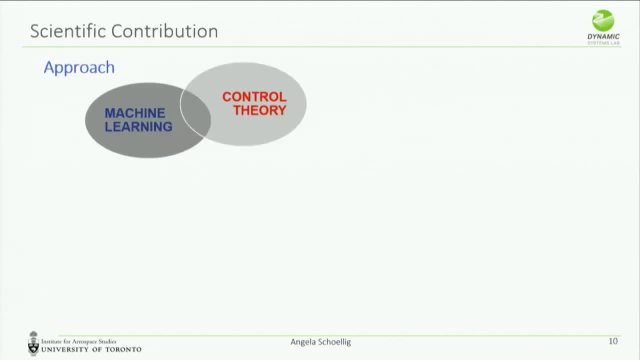 question is: what is the right learning architecture and approach for closed-loop systems? And I don't think it's really answered yet. So the approach that we have been taking over the past few years is combining machine learning and control theory, which is the 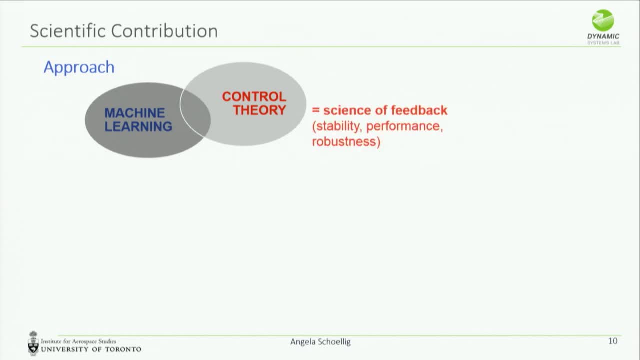 theme of this conference, which is great, And, in my opinion, control theory is really the science of feedback, So it's the only science that looks at these closed-loop systems and analyzes and defines stability, performance and robustness. And then, on the other hand, 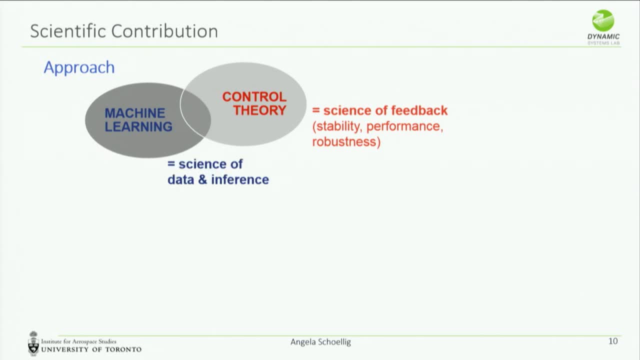 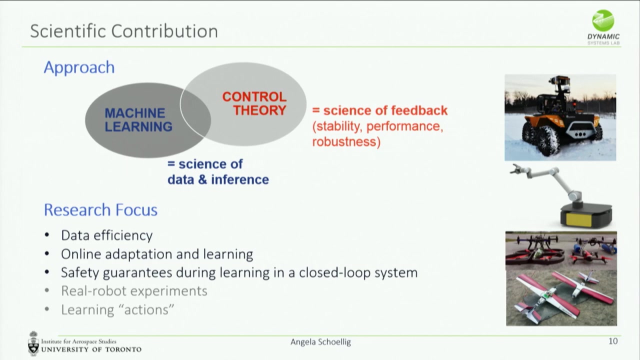 we have machine learning, which is the science of data and inference, And both together are powerful combinations to tackle some of these problems. The particular focus of our group has been because we work with real robots in the real world on data efficiency, because we operate these robots and every data point costs money. 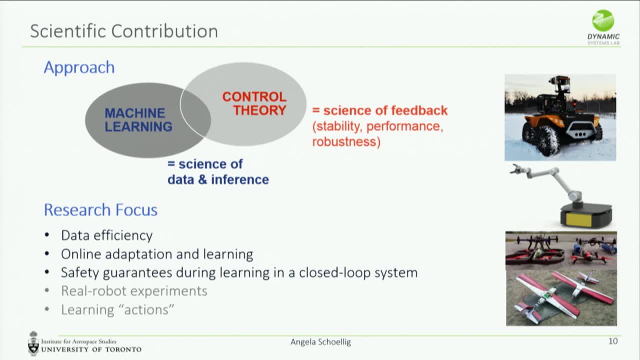 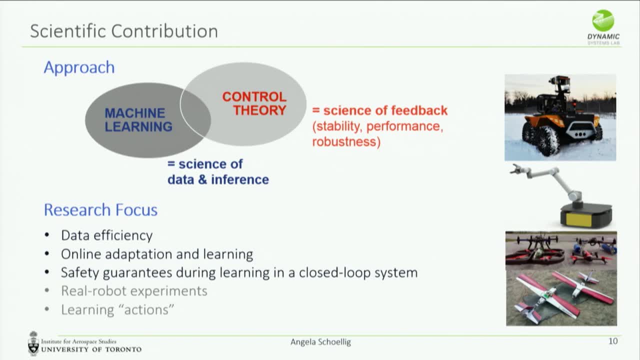 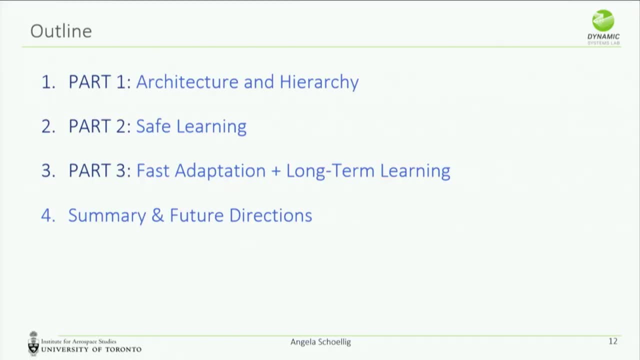 traumatic, to kind of destroy them. So what I thought I am going to do in this talk is kind of just highlight three themes of the research that I found where I can show you how control theory and machine learning can nicely work together, And so 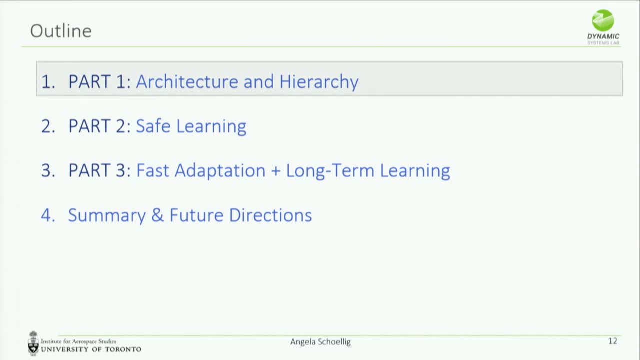 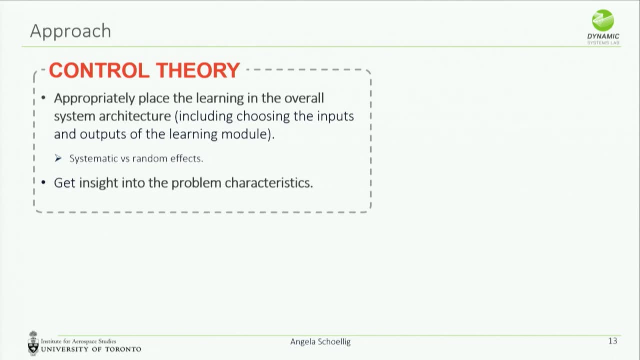 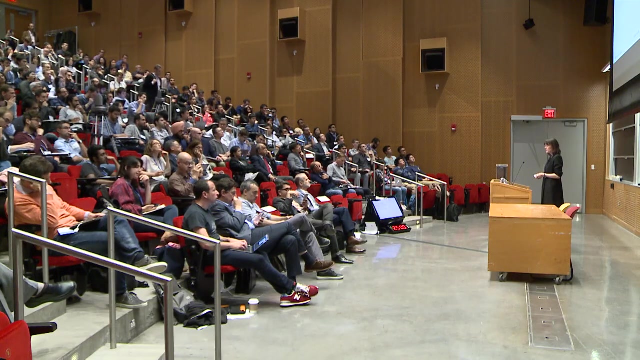 the first one is architecture and hierarchy, So control theory has helped us a lot in appropriately placing the learning in context, the overall system architecture. so control theory and generally system dynamics, allows us to understand the system. even if the system is complicated and we may not be able to identify all the components of the system, it gives us. 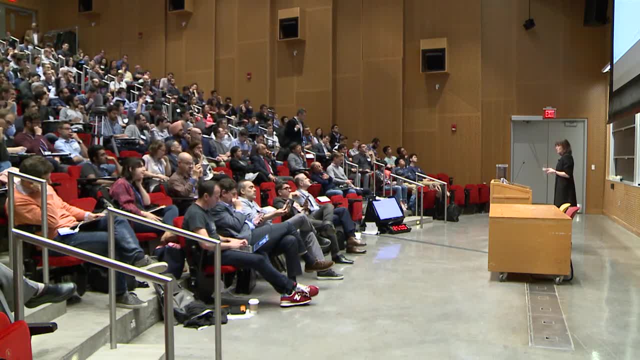 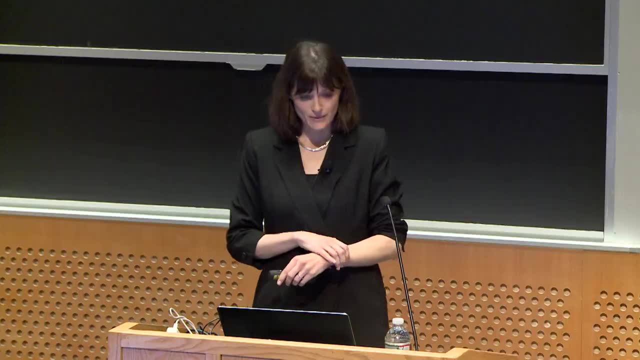 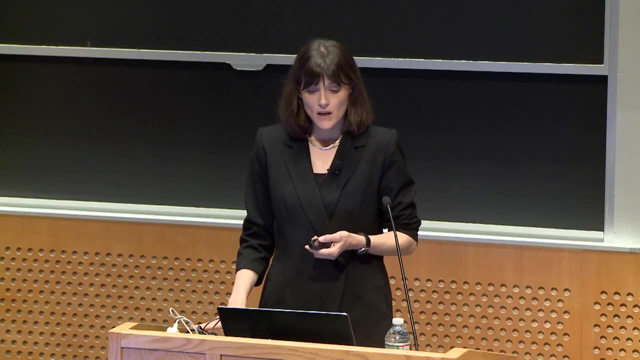 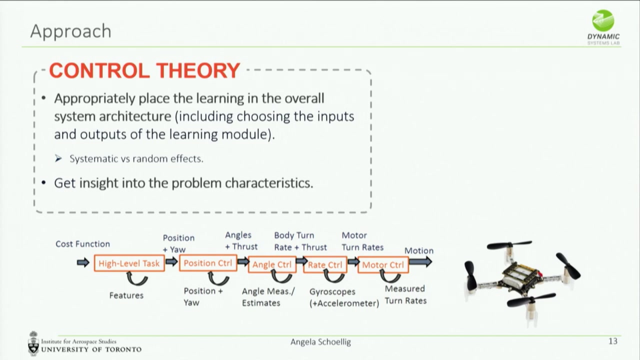 an understanding, and especially an understanding of systematic versus random effects. there's systematic effects as things that a learner can nicely learn from data, versus random effects, where the best thing you can do is really doing fast feedback. and then, as an example here for flying vehicles, you have these kind of nested control loops, starting with the lowest control. 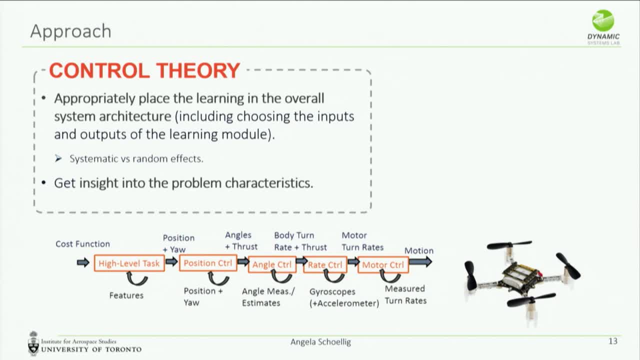 loop, which is motor control. so the motor controller just makes sure that the motor spins at the turn rate that you want it to spin, and then at the highest level. if you kind of close all these nested loops, you have position control and in the middle there's a controller that makes sure that a turn rate around 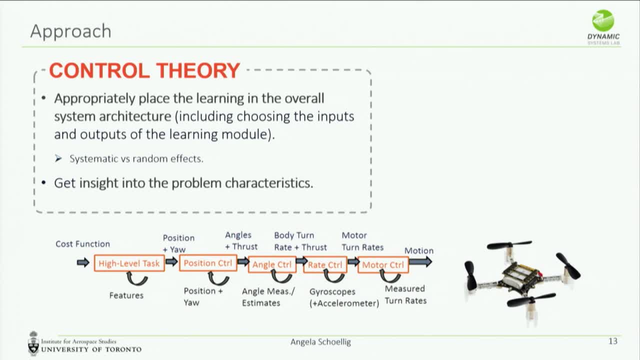 a body axis is achieved, and so in by kind of closing the right number of loops to make this to account for the random effects with feedback we have kind of a repeatable input-output pattern that is then easily learnable in machine learning, and I think that's kind of a nice way to come where both control theory and machine 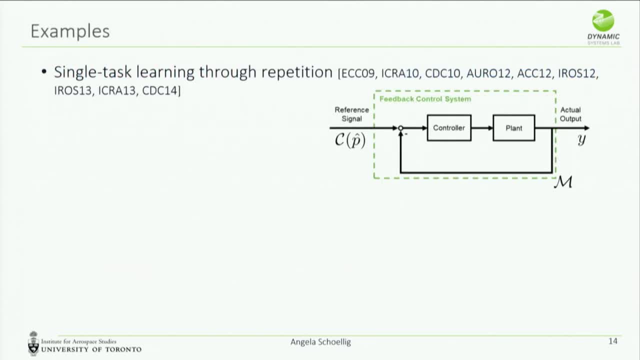 learning can complement each other. so one very early example that we did is a robot learns a single task through a repetition, and so there we close the feedback loop such that the system is stable, and then we learn the reference signal, the input signal, such that the output does what we want it to. 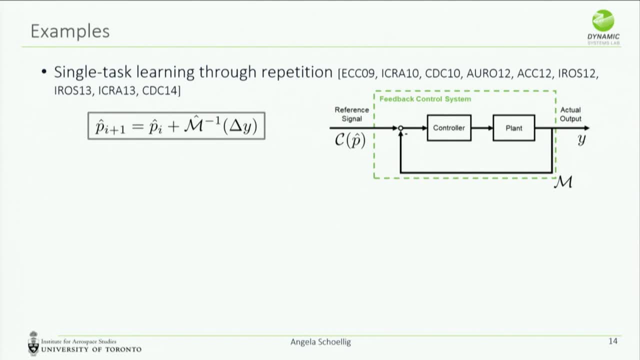 do, and so the very basic idea is that you do run the experiment, you see how much the actual output deviates from the desired output, which is Delta Y, and then you use a rough first principle model that relates this output error to a change in parameters, and so you change the parameters of your reference signal. 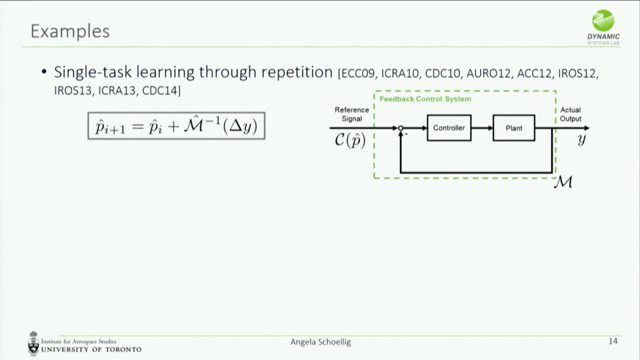 iteratively in the right direction to eventually get good performance. and so we did this on flying vehicles and did this s-shaped desired trajectory. and if we learn the desired turn rates as an example directly, we can learn that and we can. our learning converges. but the result is that after the reference, 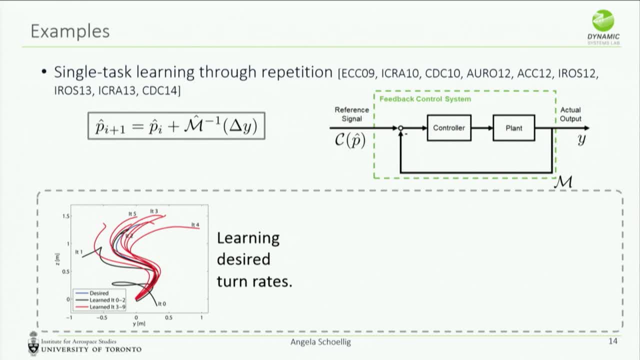 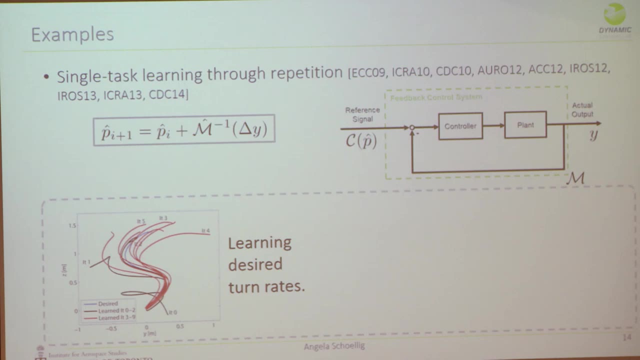 input converges. we, and we apply this reference inputs repeatedly. you see the red lines and they are not, you know, not a nice s-shape. and the reason is because we didn't close enough lower level loops, such that there's still too much randomness in the system that the ultimately 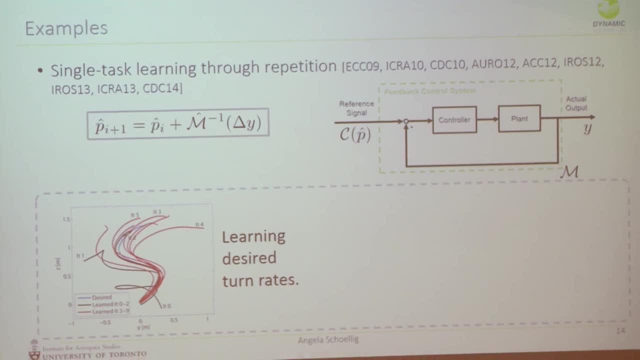 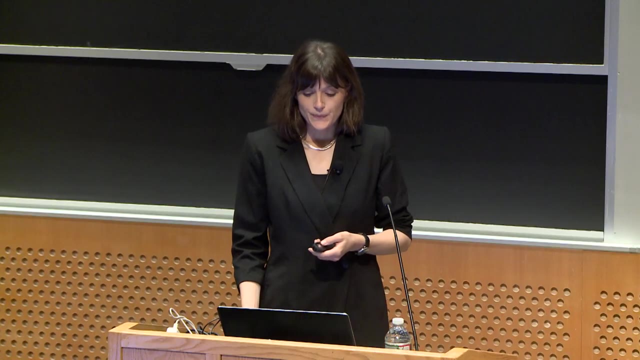 performance that we can achieve with our learning controller is not good, but if we instead do this on desired position, so we learn desired positions and no feed forward, which, because that was kind of the configuration that provided us the best and the most repeatable behavior, then the learning can actually converge. 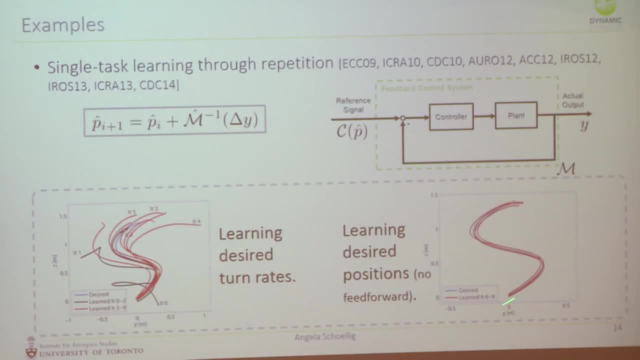 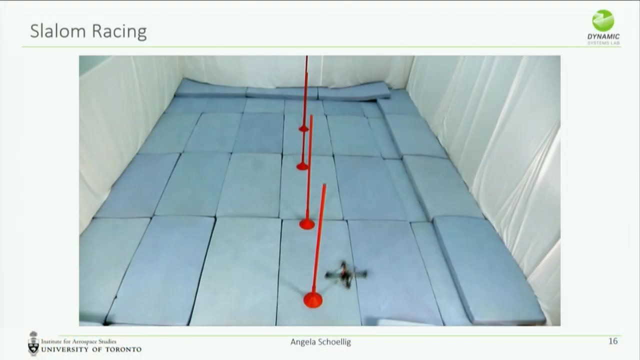 and the converged reference position input leads to a read repeatable behavior in the output and we nicely follow this s-shaped trajectory. so we use that for slalom racing and in this case, if you don't use learning- and there's quite a lot of unmodeled aerodynamic effect- it really doesn't. 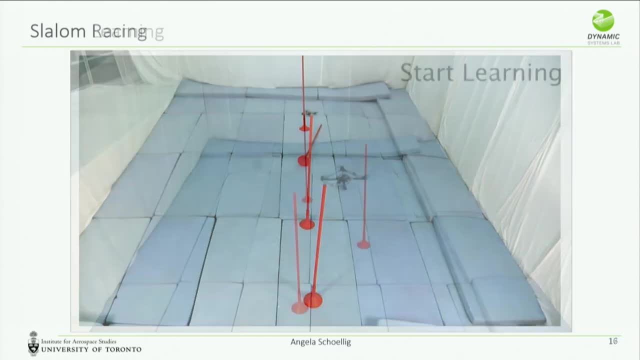 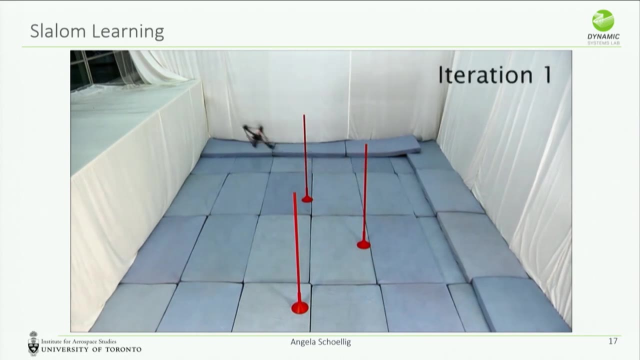 work as you would hope, and so we use exactly the technique I described, and because we close all these underlying controllers, it converges to the very quickly. and the other reason for the quick convergence is that we use our prior model information as a gradient in the learning, and so after three, 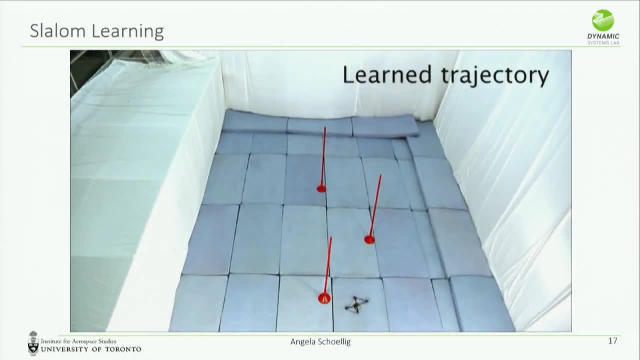 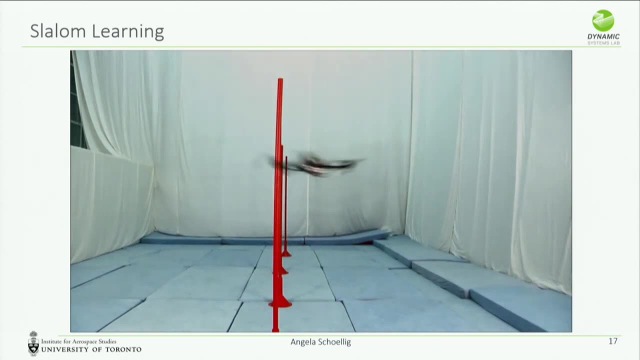 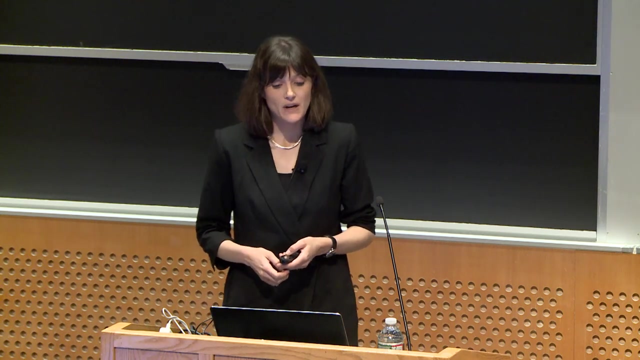 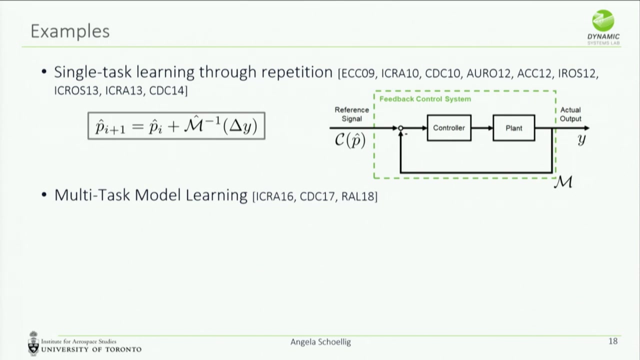 iterations. we can actually do this and we can learn arbitrary configurations, but this was a task, dependent learning, so every configuration needed to be relearned. so we thought about- and I did- that we can learn a model instead, and learn once this model and use it for. 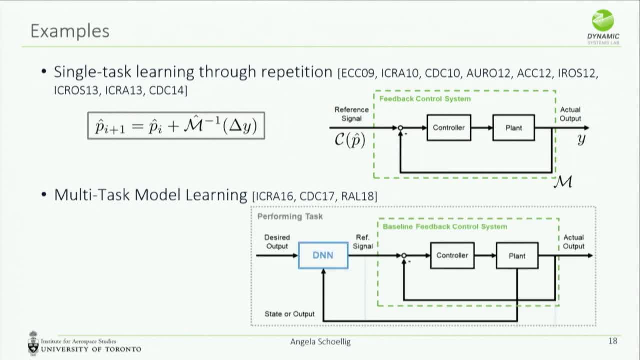 any arbitrary trajectory and the setup is quite simple. we just put this pre block there. we use deep neural network in this case, but you could use another nonlinear regression technique. and basically this: this neural network needs to approximate the inverse of the dashed green box. and we showed- and again from control theory, we can kind of quickly. 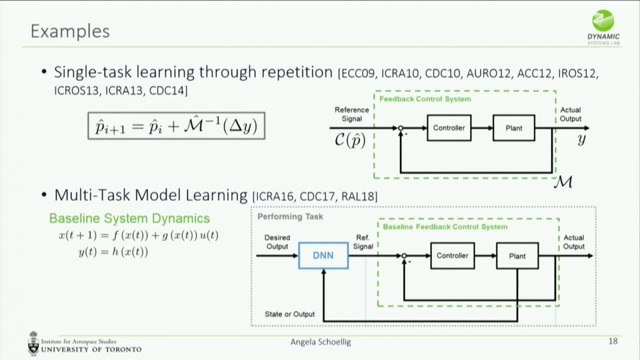 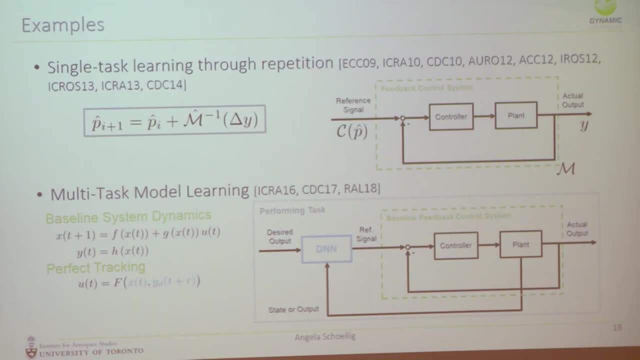 get insights. so if this, even if we know nothing about this dashed green box, if it's kind of a generic nonlinear system, if we do the inverse, we would know that what would need to sit in this blue box is this function f, which is dependent on the state and the desired 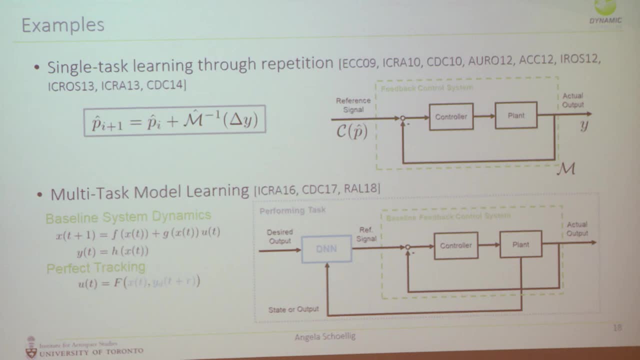 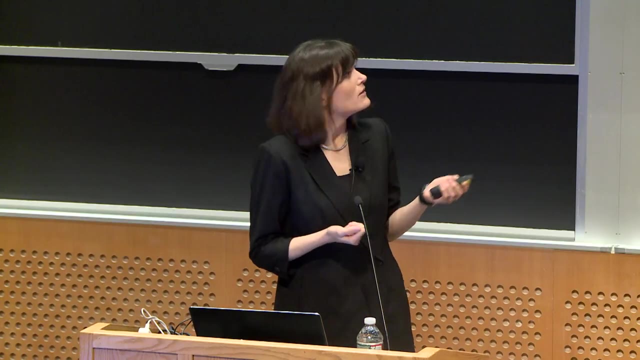 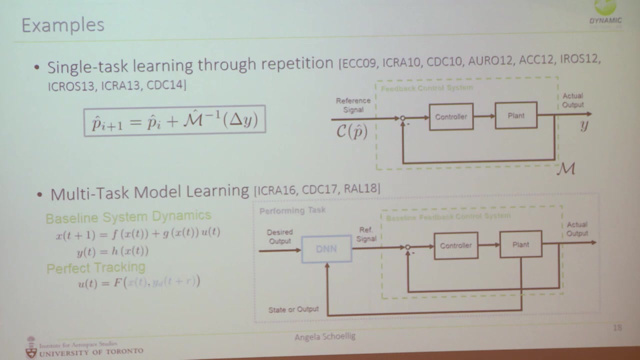 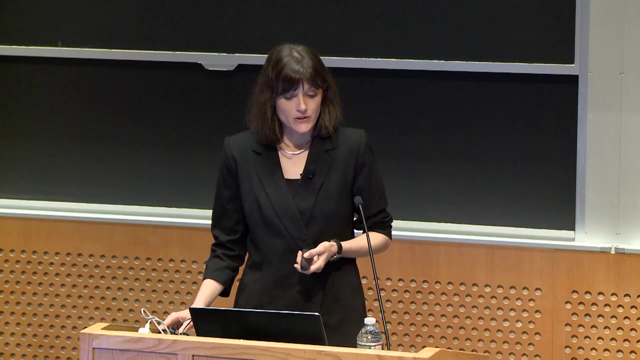 output. R steps in the future and R is the relative degree of the system. so the control theory, even if you know nothing about the system, can tell us what roughly needs to sit in this black box, in the screen blue box, and and help us to choose the right input features. and so those input features are relatively easy. 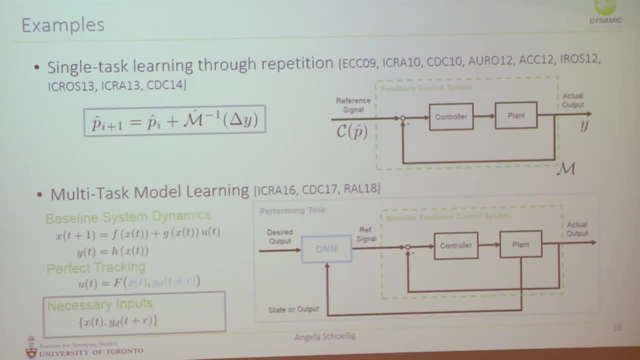 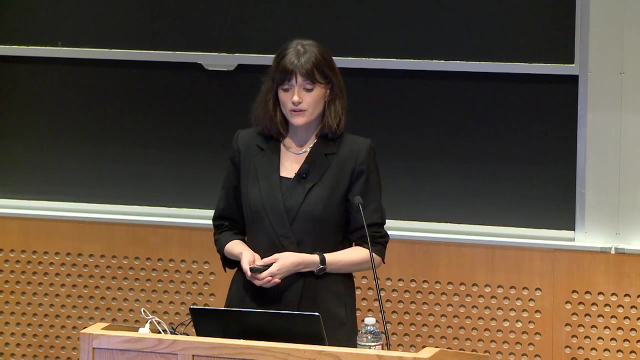 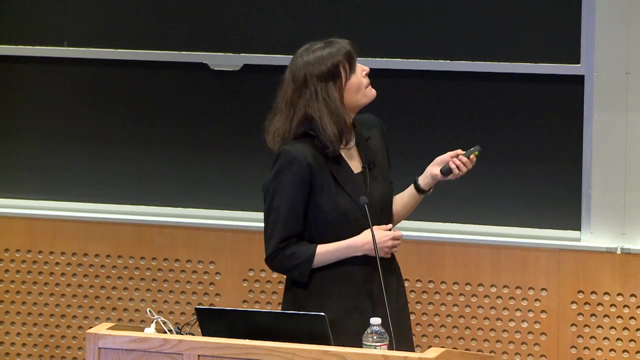 to get and if you don't know R of your underlying system, you can do a quick test like a step response experiment to get this value And go from there and learn much more efficiently than thinking you need any more input features. The good thing is we learn this box. 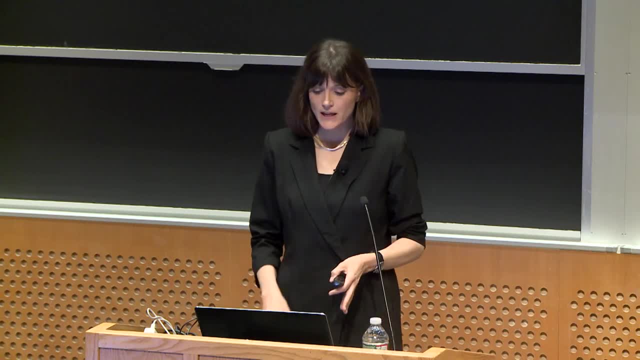 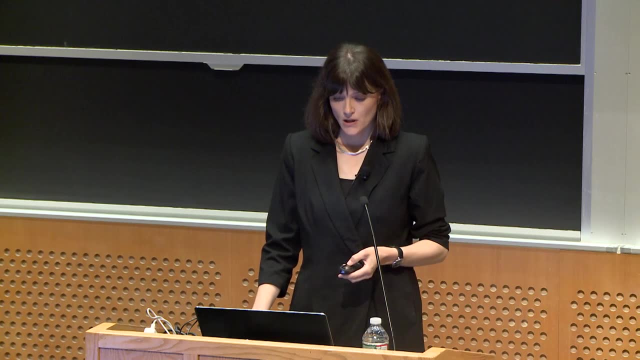 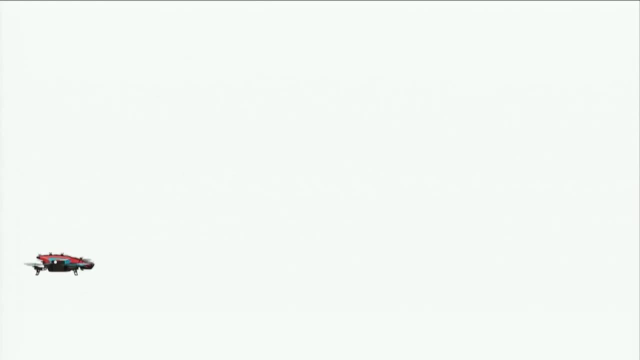 from a number of trajectories, and then we keep it fixed And we can be better in tracking any new trajectory, And so here's an experiment. The idea was that you can draw something on the tablet and that the controller follows, And this is the performance of our standard controller. 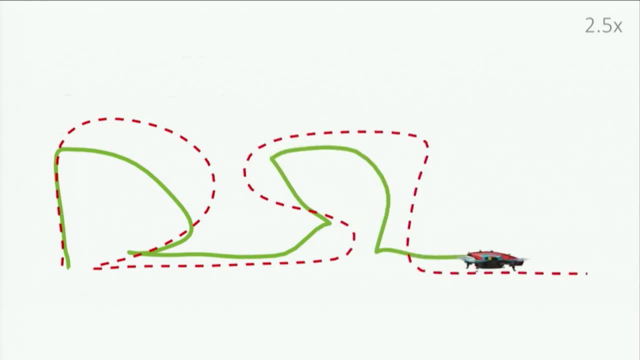 It's not great. There are many non-idealities in the system. And then we add this learning block and the tracking of this red dashed line gets much better. So usually, Usually, we have a performance improvement of over 40 percent. 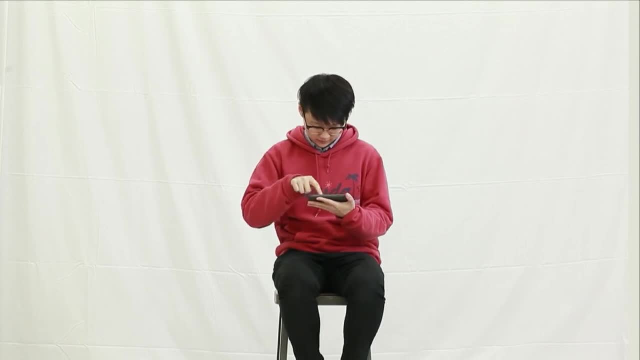 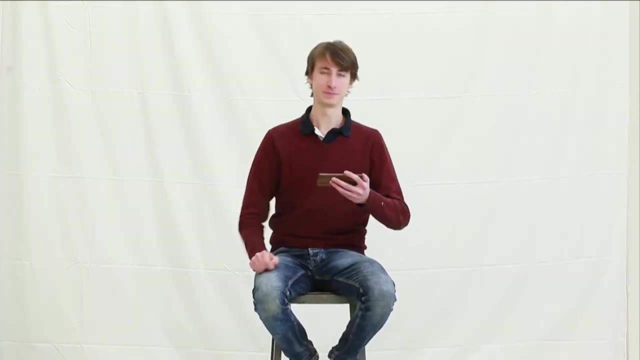 And so we did a lot of kind of tests in the lab where people would draw different trajectories, And we know from control theory that a standard controller would not be able to perfectly track any of these trajectories, even if we would know the model perfectly. 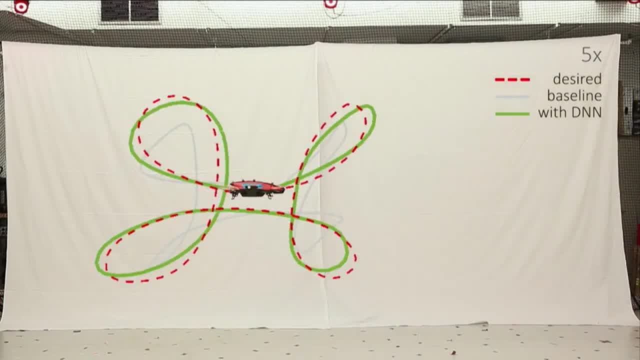 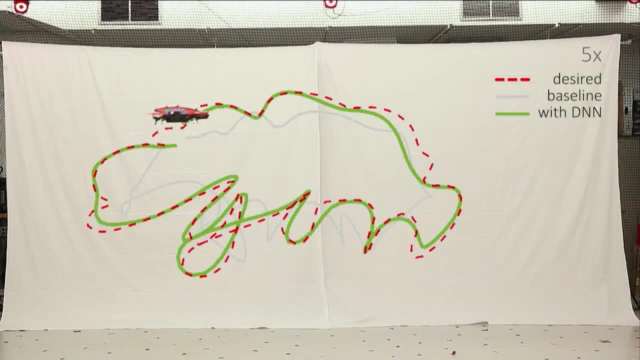 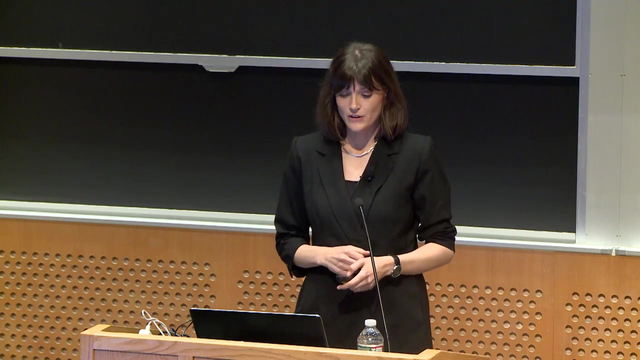 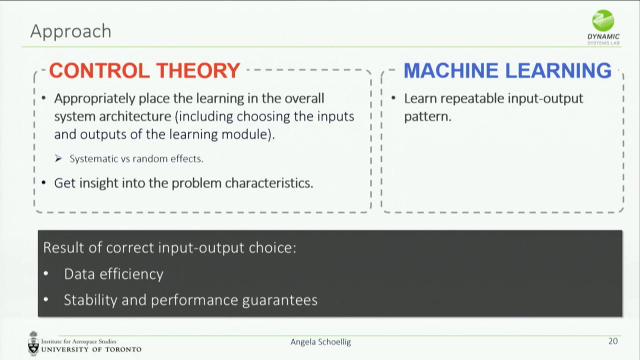 And so you see that the performance is improved even for complications, And that's why we have these data drawings. So, if you look at this idea of architecture and hierarchy, what it really helped us is that control theory told us where to put the learning in the closed loop. 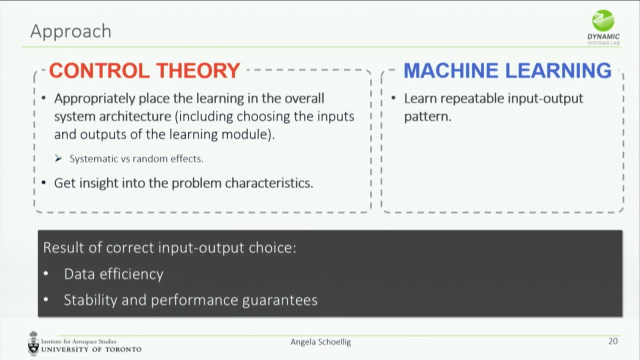 And this helped with data efficiency and also with stability and performance guarantees, Because, as you saw, the learning was always outside of the inner loop, So we could make the inner loop stable And as long as the output of the learning system was stable. 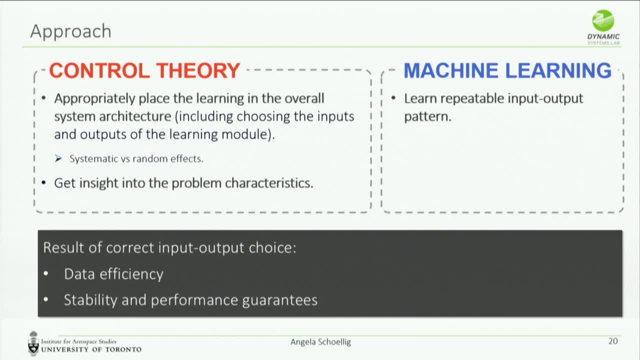 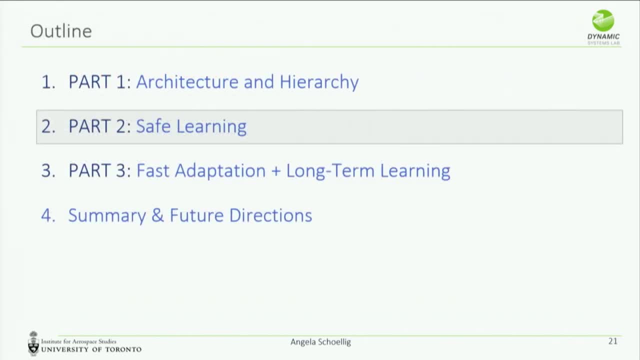 and the learning system is bounded. we have at least bounded input, bounded output stability. So I think there's lots to explore there. These are just two examples of how you could play with where to place the learning in the overall architecture- Another interesting area we have been working on. 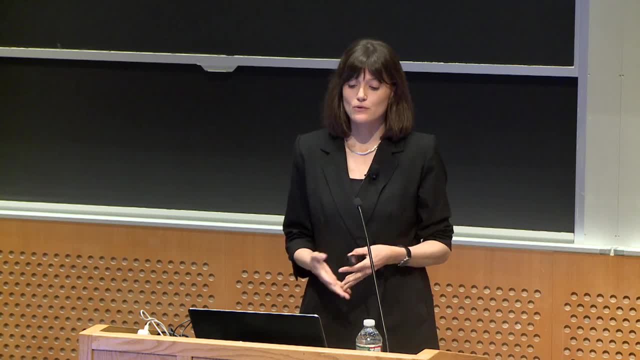 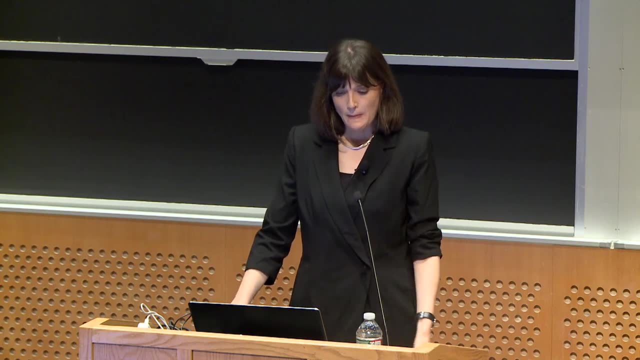 is: how can we achieve safe learning If we drive these robots outside? we want to get them out. We want to get them out, And then we'd have a very stable learning as well- and at the same time, guarantee with high probability that they don't crash. 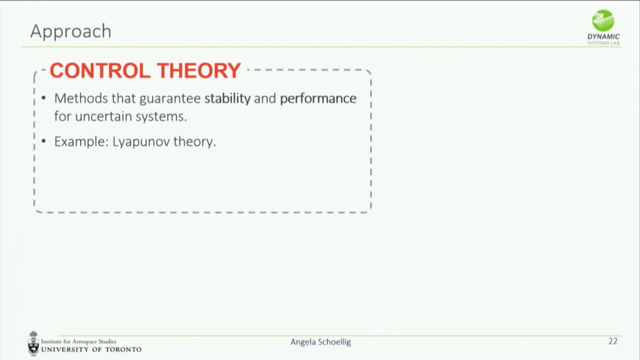 And so control theory has really nice methods to guarantee stability and performance for uncertain systems. That's robot's control theory. Usually these uncertainties are fixed a priori, And then they use techniques such as Lyapunov theory to prove stability. On the other hand, machine learning- if we make very weak 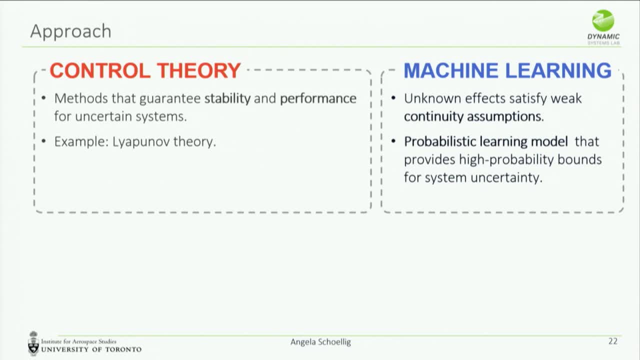 effects, such as continuity assumptions. there are probabilistic learning models, such as Gaussian processes, that provide us high probability bounds for a function, And those high probability bounds shrink as we gather more data, So this may look like this. So initially we have no idea. 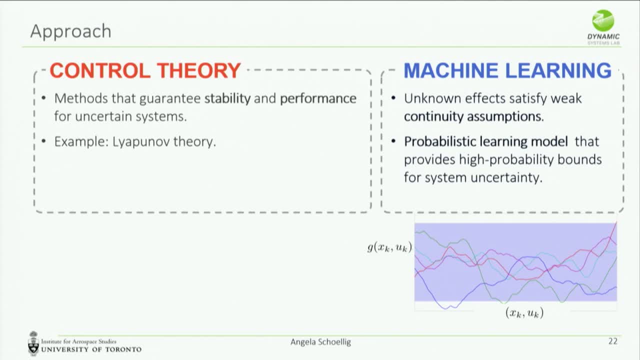 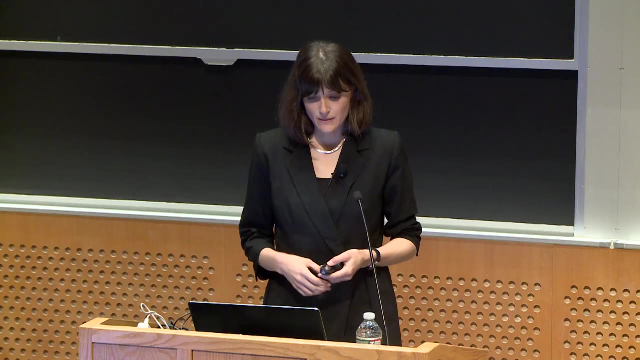 It could be anywhere in this light blue envelope. But then, as we gather more data, we get more certain in certain areas and we can adapt our controller, And so one of the first approaches that we did was that we model our system like this: 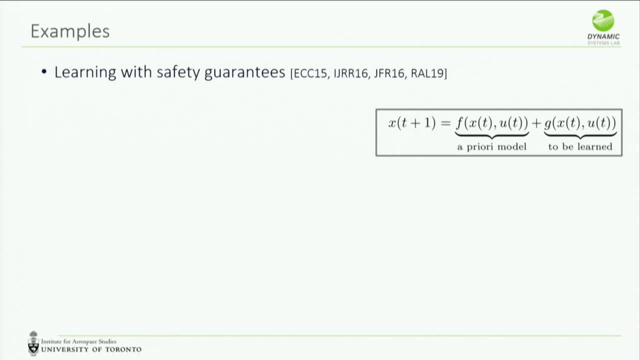 We have an a priori model which can come again from first principles, a kinematics or dynamics model, and then a model error that we are learning, And we use the probabilistic learning model in order to specify those Uncertainty bounds. 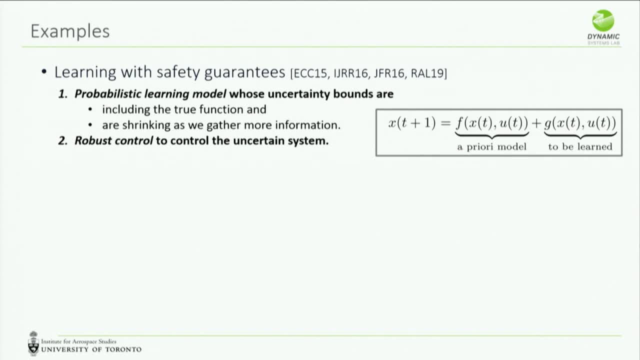 And initially we need to assume that our true function lies between the initial assumptions of the uncertainty bounds. so you can make them quite large, But then, as you gather data from the system, you learn more about this model error and you shrink those uncertainty bounds. 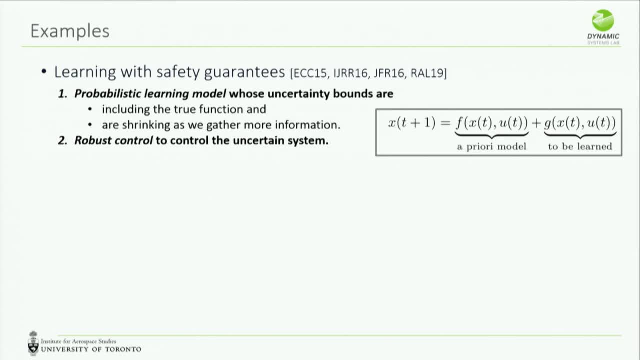 And with some formal assumptions, you can guarantee that those uncertainty bounds that you get from your probabilistic model are actually true high probability bounds for your system. And then we use robust control And one early approach that we did was we combined this probabilistic model. 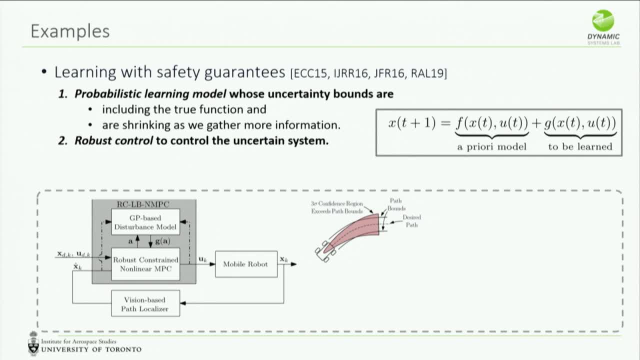 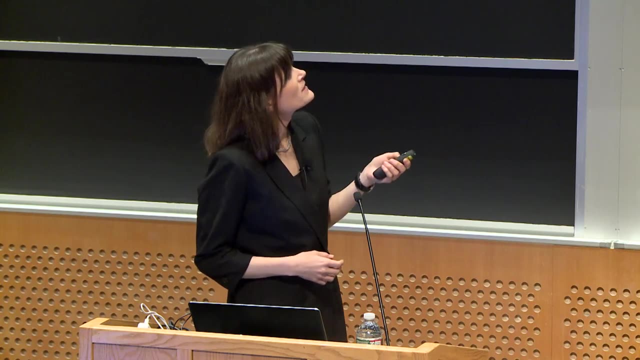 with robust, constrained, nonlinear model, predictive control for following doing off-road path, following where we want to increase the speed of the robot as it learns more about the world. And so how that works is- you can look at this picture- So at a given moment, the robot is going to be able to do this. 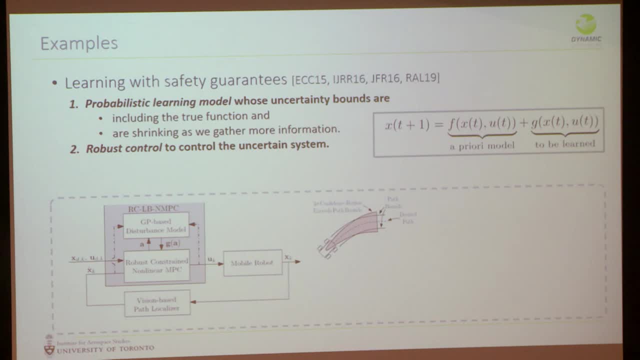 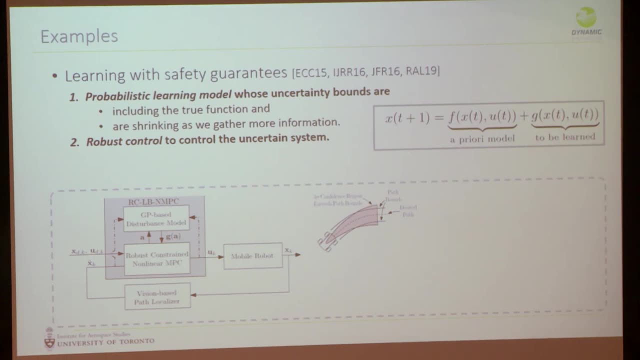 And then we can use robust control. And then we can see that the robot sits here And, with model predictive control, it uses its model to predict into the future. So for a fixed input sequence the robot may end up anywhere in this envelope. 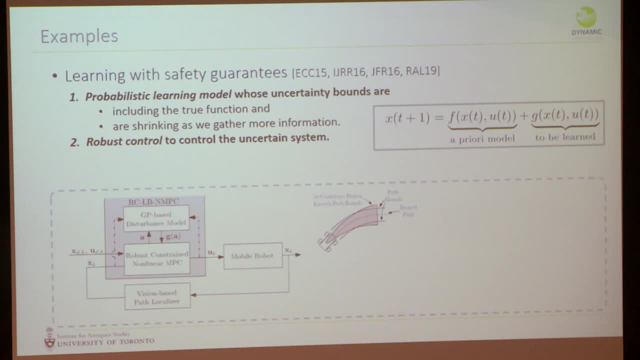 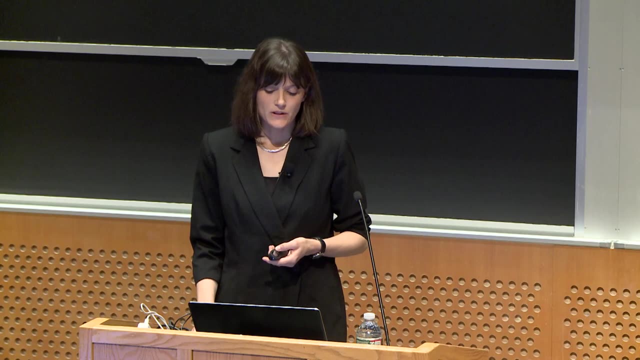 And the reason why it's ending up anywhere in this envelope is because we have this stochastic model, like the Gaussian process, which doesn't tell us exactly what the robot does Right, And so, before learning, we have to do this. We have a high uncertainty. 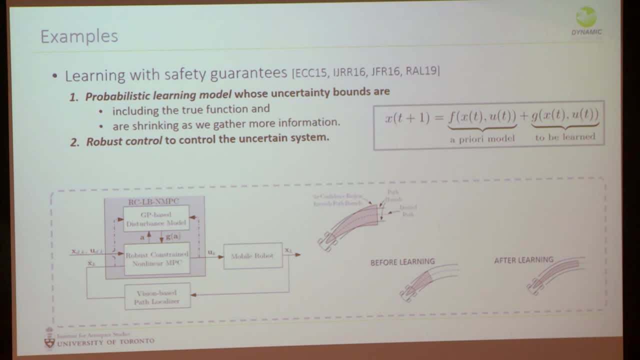 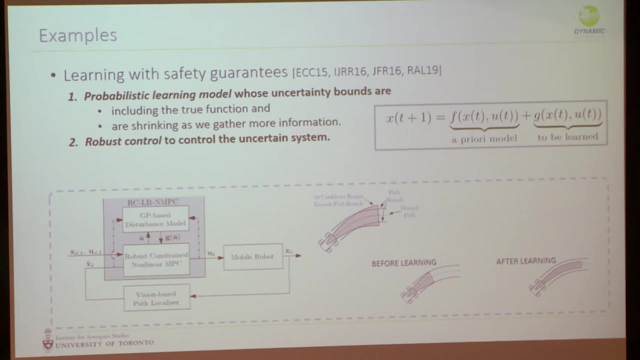 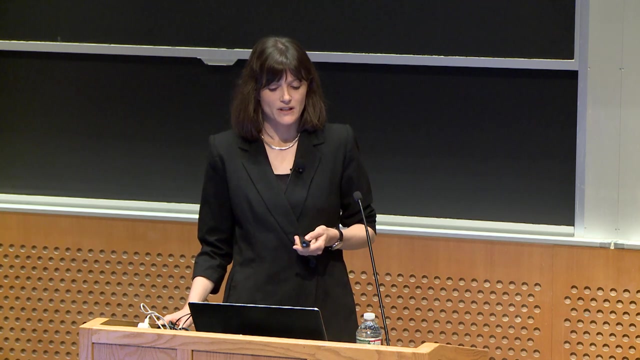 And what it does is that it reduces the speed, meaning that over a fixed prediction horizon we don't get as far, But it makes sure that we stay within the path bounds, with high probability based on our probabilistic model And then, after learning the probabilistic model, 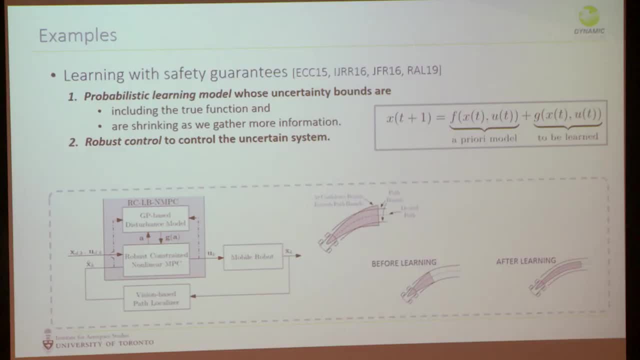 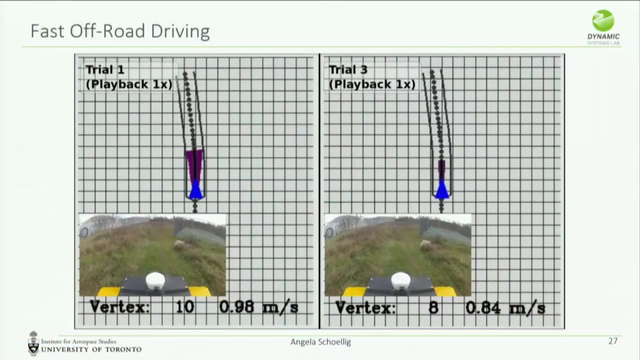 is more certain And we can try faster without getting off the path, And so we did a lot of off-road testing. So here's just one example: On the left you see the robot driving the first time, And on the right, the robot driving. 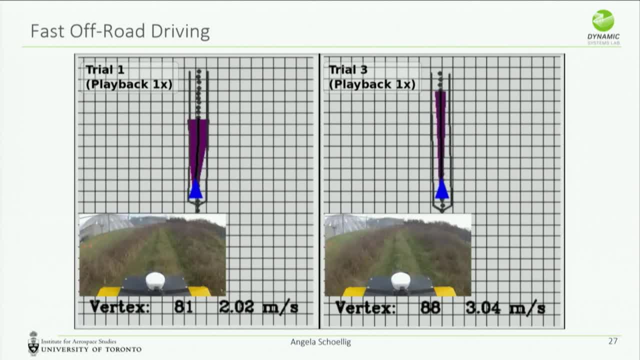 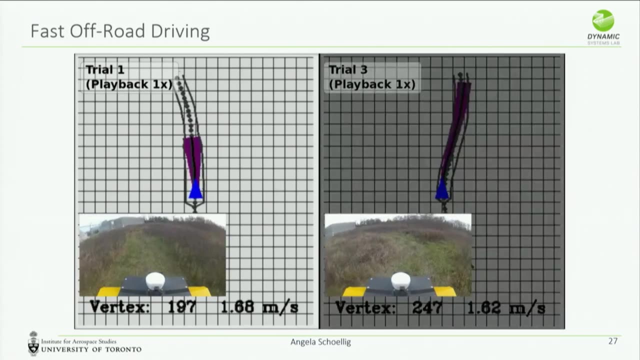 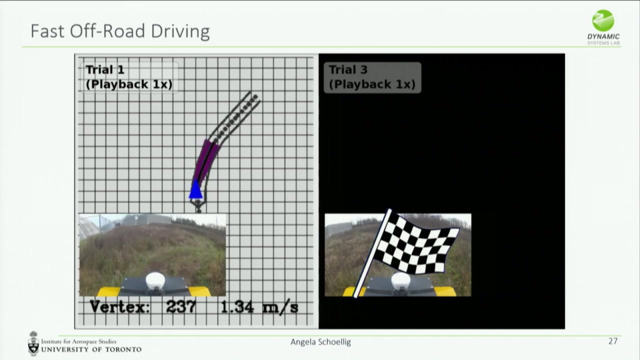 the same path the third time, And so it drives significantly faster. You see, the uncertainty envelope is smaller And we drove with this robot, with this method, faster than we have ever done without being too worried that something happens. And so it finishes this particular segment. 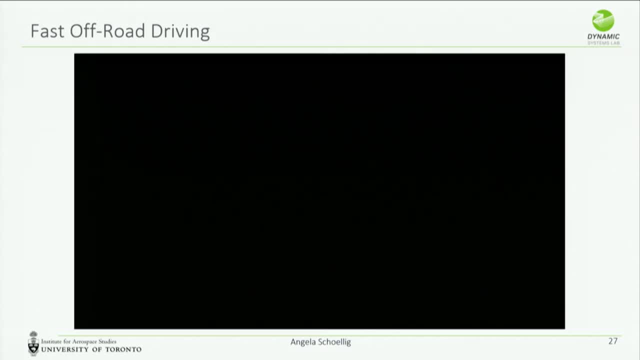 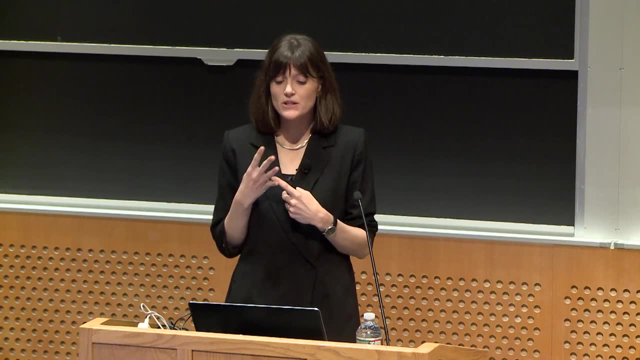 of the path faster than it did in the first round. We also tested this on four different robots without really re-tuning the algorithm. So one robot was from the Canadian Space Agency, one from Defence R&D Canada and one smaller robot in our lab. 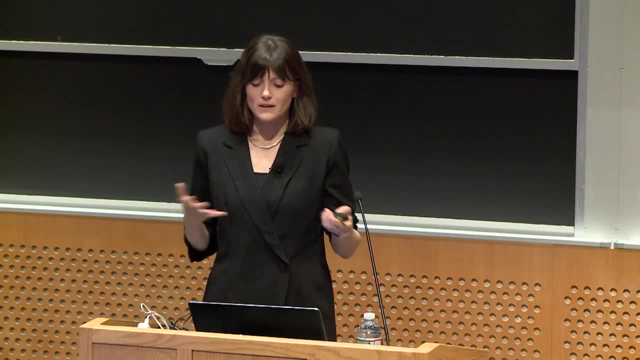 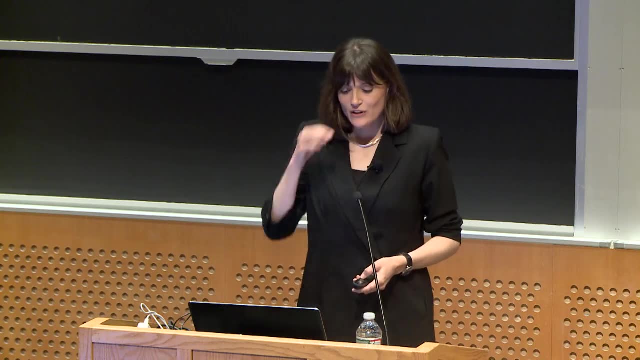 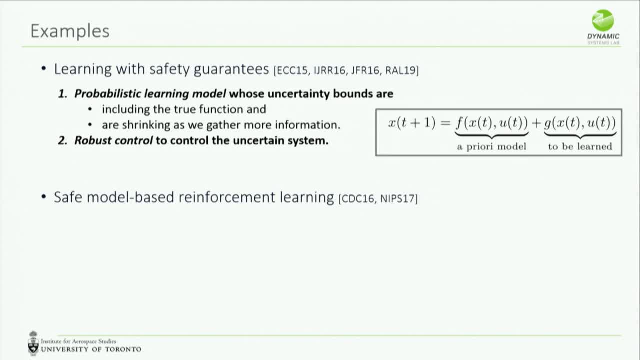 I assume that this is in collaboration with Andreas Krauss and I assume he will tell more about that, But the idea is that reinforcement learning usually doesn't have a notion of not trying out actions that very likely lead to disaster in some form, So this is kind of crazy. 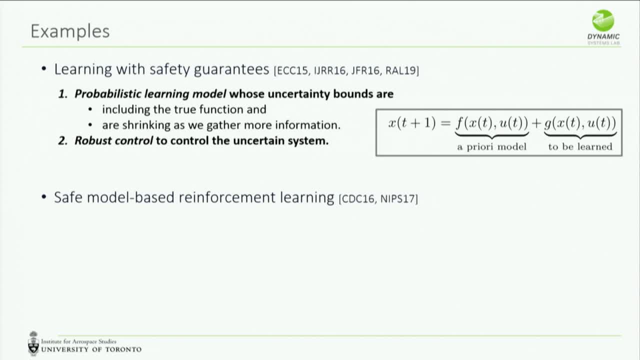 First, you try things out that on a real system. you try things out that are dangerous. But even if it's in simulation, you would think that this is not very efficient. You try things out that you know, possibly a priori, that 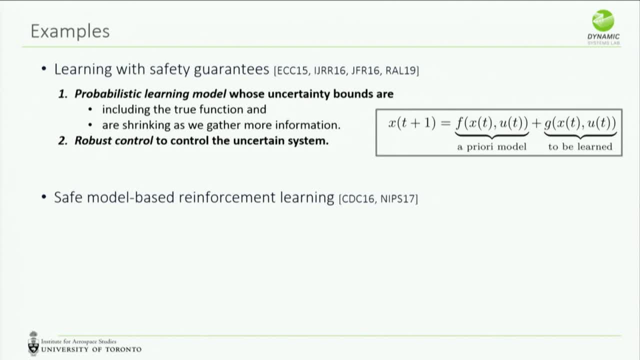 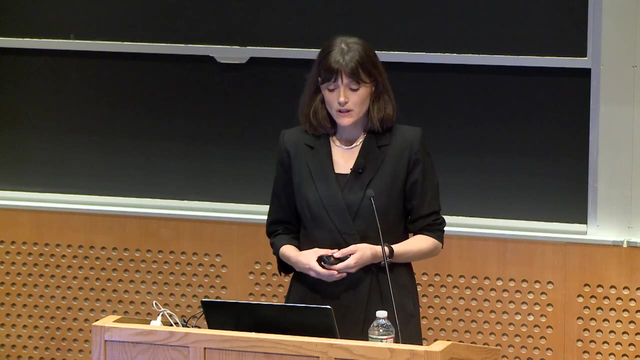 will not lead to success, So why should you even try it out? And then we also use Gaussian processes in a more model-free approach to do safe automatic controller tuning. And we applied this to tune an adaptive controller, which was really interesting because there's 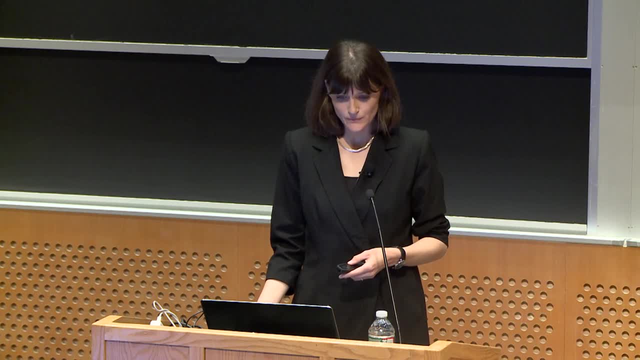 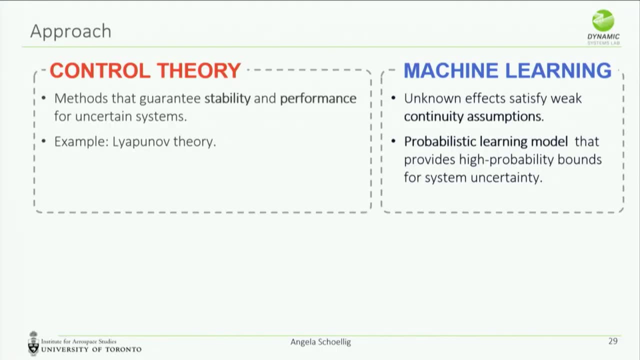 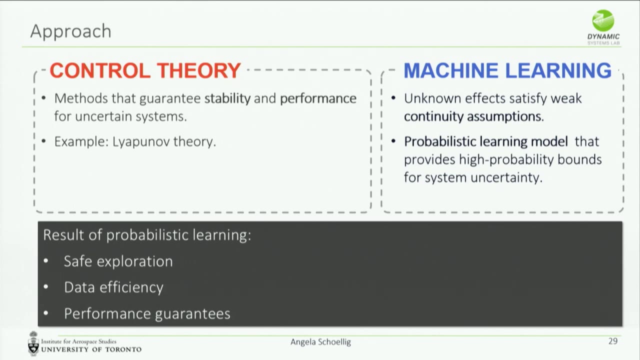 no really optimal tuning strategies for adaptive controllers. So, in summary, when we kind of combine these two techniques for safe learning, we could achieve safe exploration, under some assumptions of course: data efficiency and certain performance guarantees. Again, whenever you need to do the proofs which I 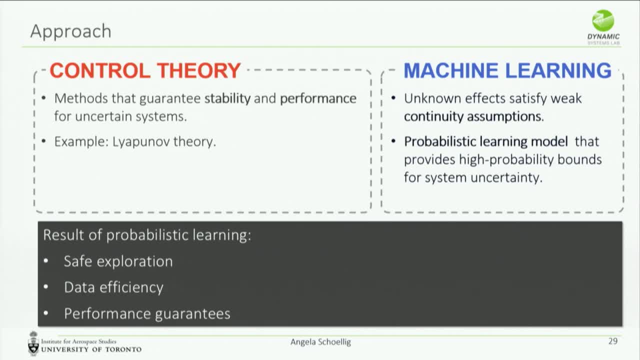 always do, And you can do the proofs and you can do the models, and the models, and the models, And if you don't do them and you don't do them, you get very weak assumptions. So when you have the things that we omitted here, 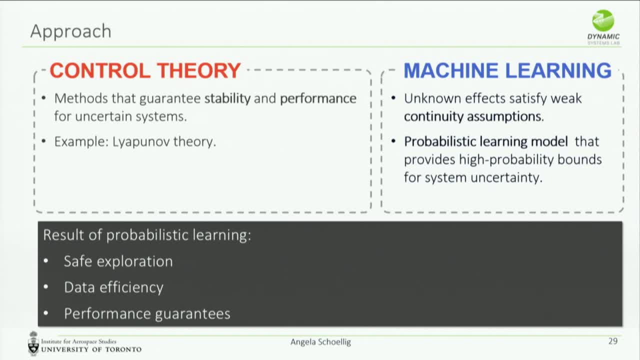 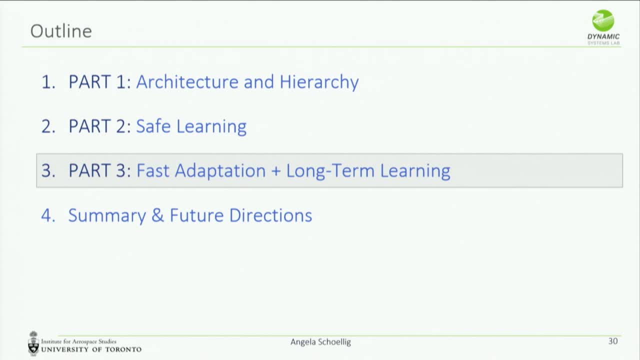 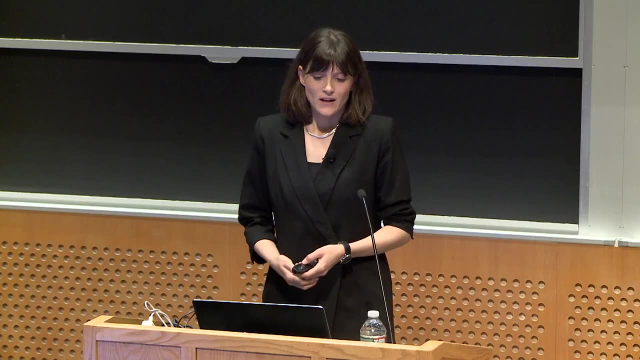 you make some very weak assumptions, But our goal is always to make very weak assumptions about the things that we don't know. So here, in this case, about the unmodeled model error or unknown model error. So, finally, the last idea is something: 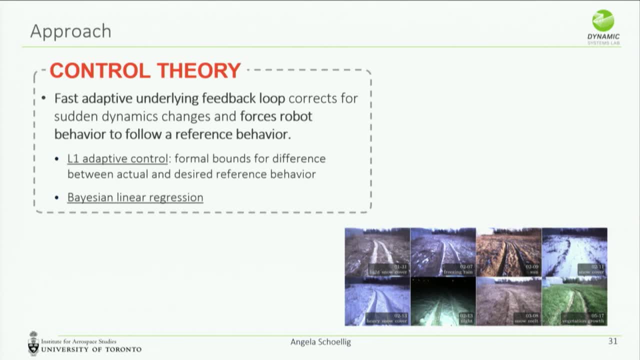 that we are very actively working. fast feedback is a really effective way to control a system, especially under disturbances, And so our idea here is: can we combine fast, adaptive feedback control to force the robot behavior in a particular way and then do high-level learning? 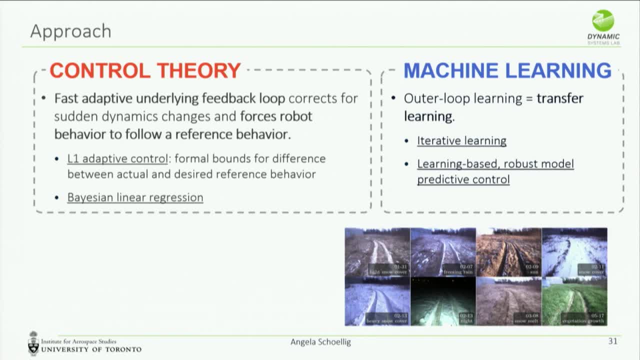 And the idea is that this is an image of our off-road robot traveling the same path over four months, and so it experiences. you know, in Canada we have freezing rain, we have a lot of snow, then at some point it's really wet. 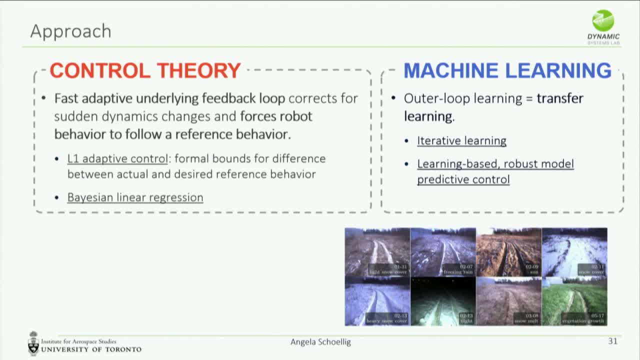 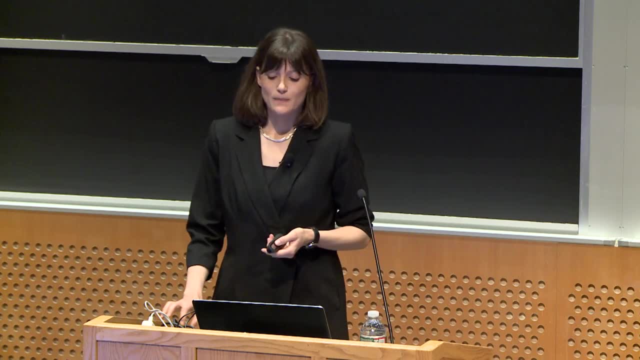 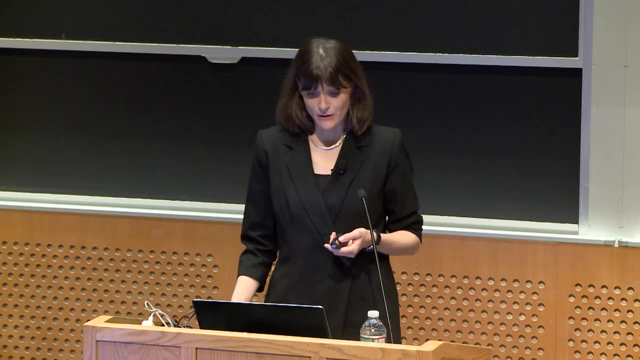 and then eventually maybe there's spring in May, And so these conditions are really hard to predict, and if the robot goes out and has never seen this condition, the best thing you can do is really really fast feedback and really adapting very quickly. 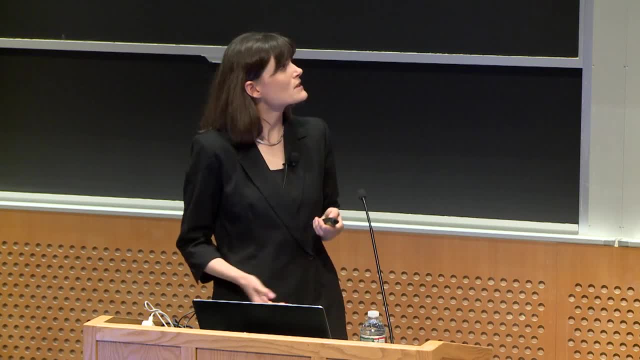 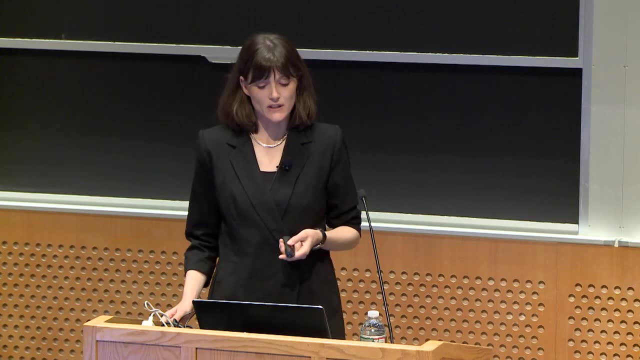 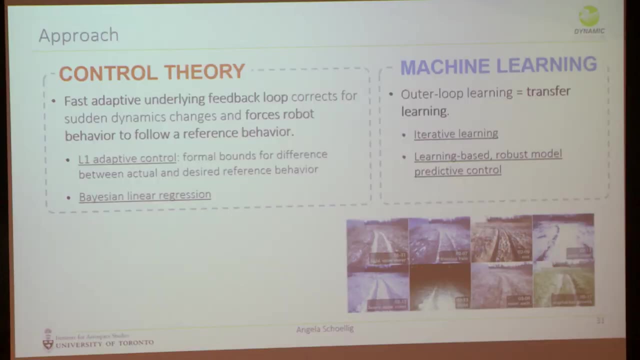 But then, on the other hand, you think that you could learn something from this winter for next winter, so you could rediscover a condition that you may have seen before. And so, on the control side, we looked at L1, adaptive control, because it allows or provides some formal bounds. 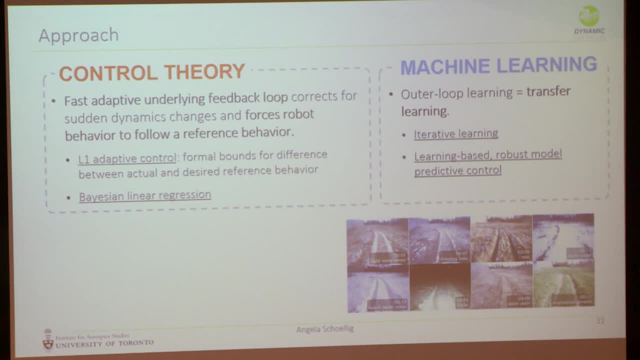 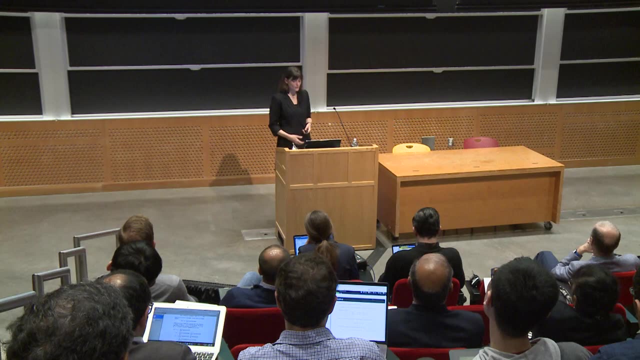 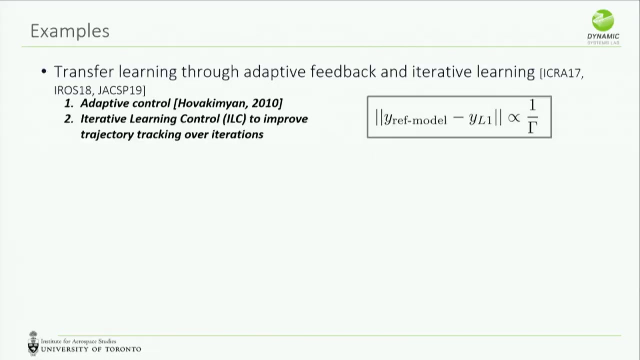 of the difference between the actual and the desired behavior. And then, on the higher level, we used techniques that you saw before, Similar to the slalom learning or the off-road robot, And so adaptive control, especially this L1 adaptive control. it provides you a bound between the output. 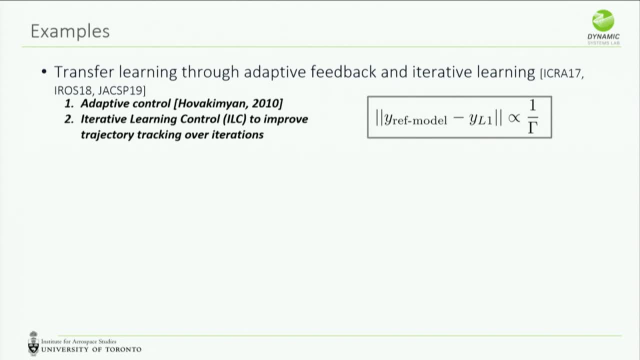 of what a reference model would do, a reference model that you specify and the actual system under the L1 adaptive controller. And this difference is bounded by the L1 adaptive control, So you can specify a function that's proportional to 1 over gamma, where gamma is an adaptation gain. 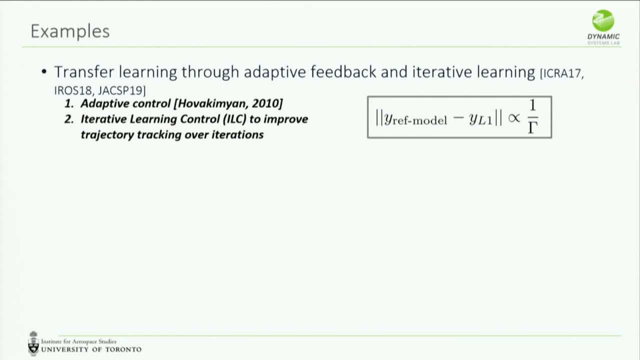 that you can choose very large, So you can make this difference small, And so what that means is, if you put this adaptive controller at the lowest level, the dashed box performs very closely to a reference model that you specify, which could be some linear or second order system. 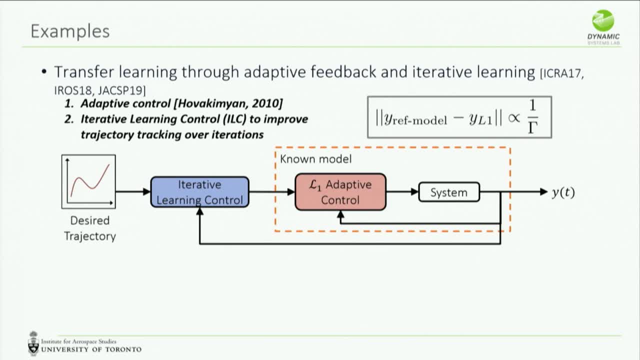 And then you can put on top something that further improves the tracking performance or does some other higher-level learning, And so if we do that, then the goal is that, in our case, a simple goal is that the desired trajectory matches the actual trajectory. 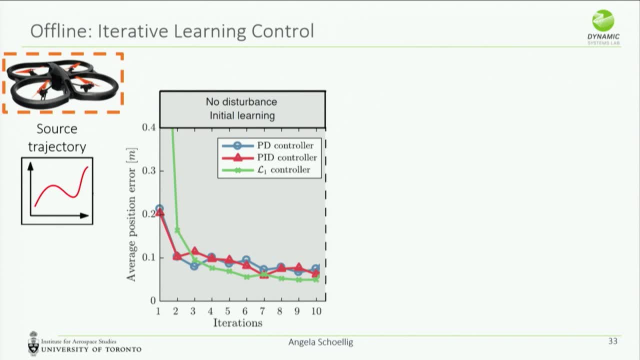 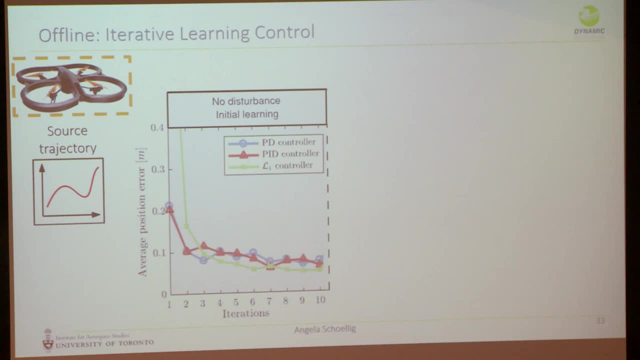 And so, as a first test, we tested it on a flying vehicle. Here you see the flying vehicle doing a certain task multiple times, And on the y-axis you see the average performance. And so as it does the task multiple times, it gets better. 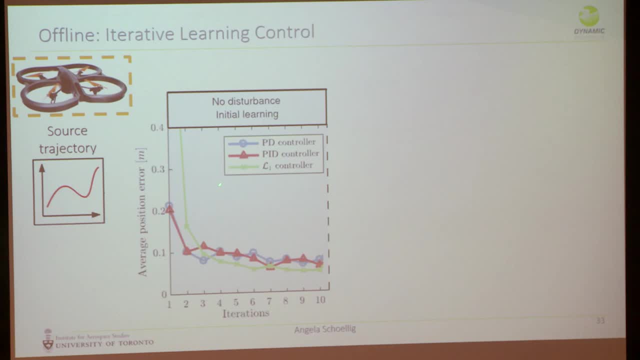 similar to the slalom learning, But we do it for different underlying controllers- a PD controller, PID controller and this L1 adaptive controller- And then we introduce a wind disturbance And that's what we see. So we introduce the wind disturbance. 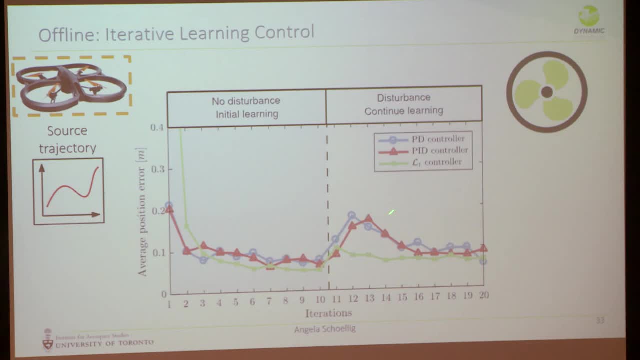 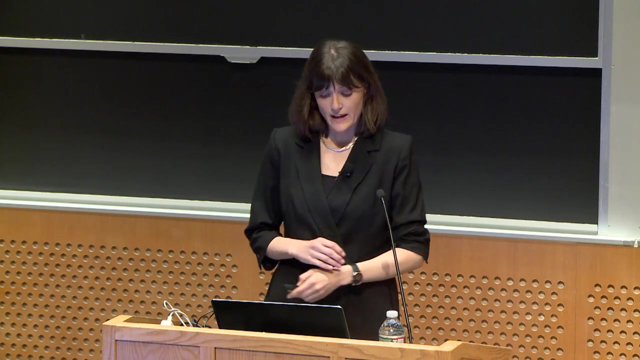 And basically for PD and PID. this higher-level learner needs to relearn. but with the adaptive controller? the adaptive controller takes care of the wind disturbance and the high-level policy can be reused. So the adaptive controller really handles the disturbance. And then we were wondering: can we even use that to try it on a different system? 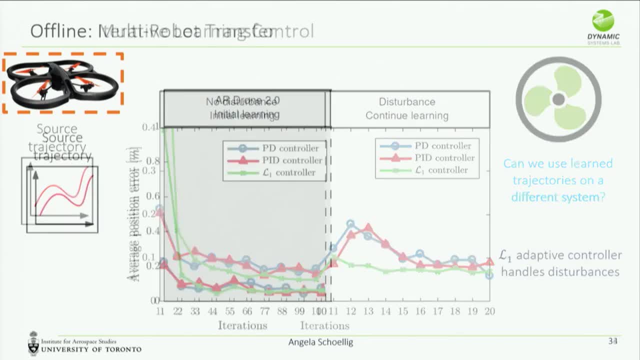 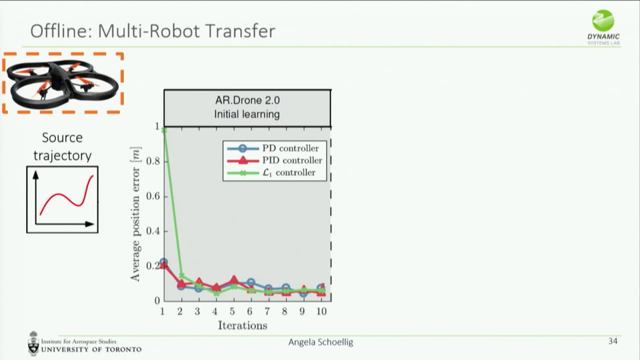 like transfer from one robot to another robot, And so we did some first experiments. We are in the process of doing and analyzing this more- where we transfer this knowledge to a similar system, Similar but different robot, different in weight, different in the inertia values. 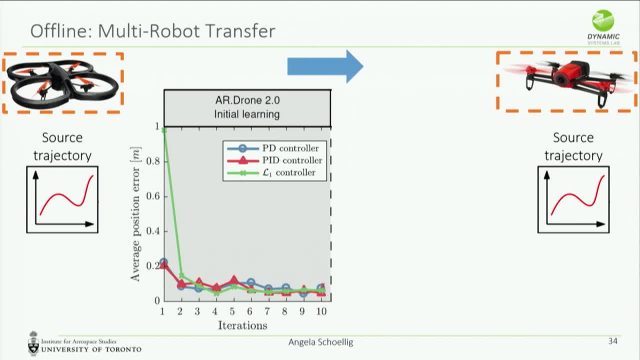 And here we try to do the same task with both of them again, And these are the results. So again, really, the high-level learned policy can be readily used again, because this L1 adaptive controller makes those two systems basically look the same on the higher level. 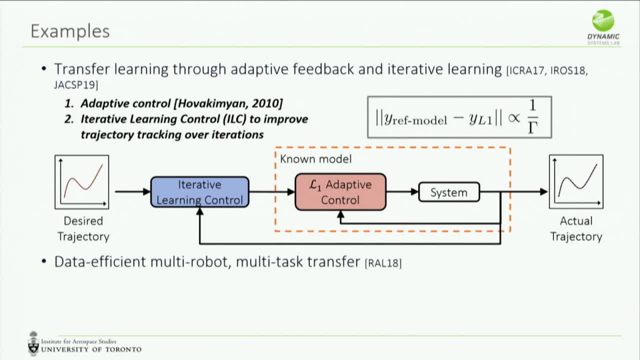 So that was it. It was quite promising. And then we recently extended this work to learn with one robot a task A and then use that knowledge to do task B with another robot, Again relying on this underlying controller, and this actually works really well. 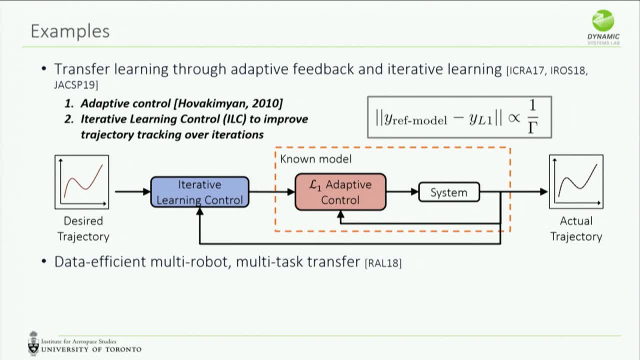 and it's very simple: multi-task, multi-robot transfer with very, very little data. And another very recent result: It's very, really store for this off-road robot any data point that we get and do, on the one hand, fast adaptation with patient linear regression and long-term learning. 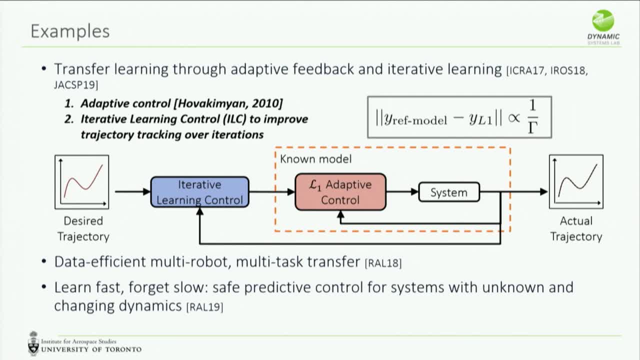 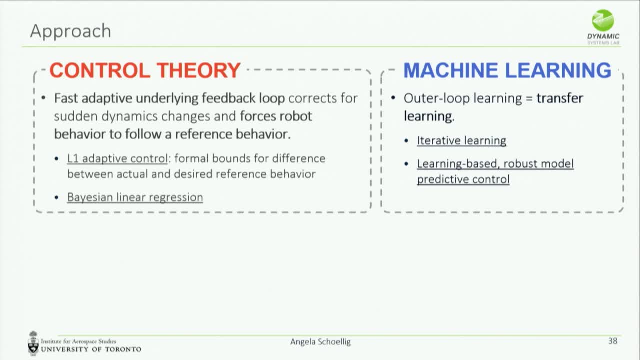 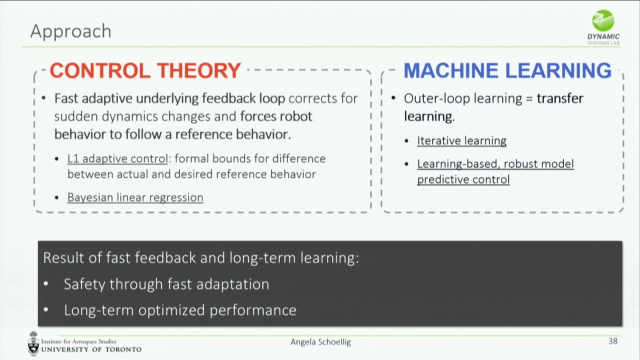 to improve our predictions of those systems. So, overall, by combining this very fast underlying feedback with high-level learning, we could get safety through fast adaptation And we can long-term optimize our performance. And we work both on more formal proofs, especially for the last work I showed you. 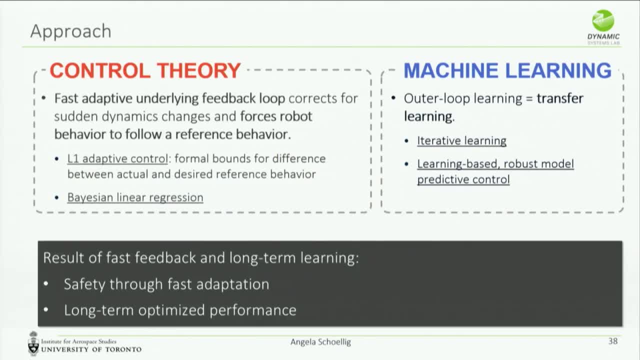 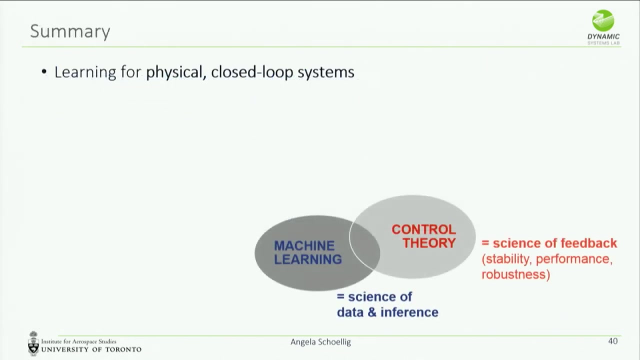 the learn. sorry, oh, what am I doing? Anyway, we work on formal proofs for some of these and have proofs for simplified scenarios for other techniques, So you can look at the papers for more details. So, in summary, you know we in control theory, we should be concerned about learning. 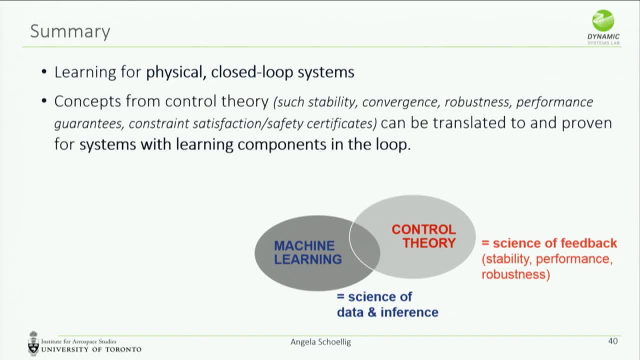 for physical closed-loop systems And I think the concepts from control theory are really relevant and interesting to analyze for learning systems and concepts like stability, convergence, robustness, performance guarantees- all these things have been defined in control theory and are not necessarily the same. 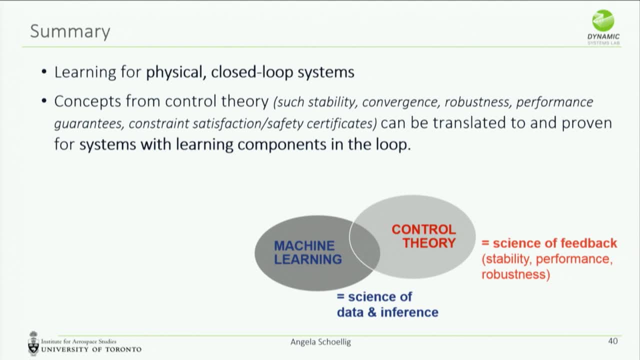 And they're not necessarily known to people in other communities. And then, in our case, we showed for some very specific cases that we can be very data efficient, achieve online adaptation and safety guarantees during learning by combining machine learning and control theory concepts. 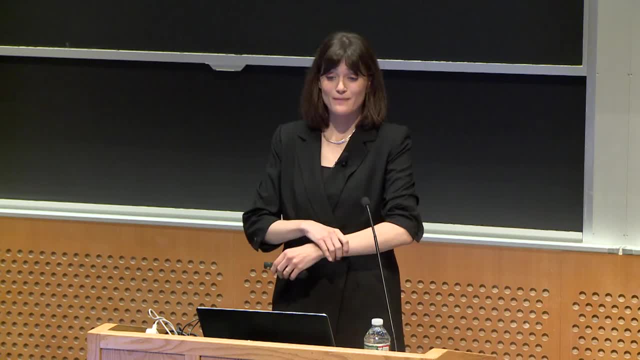 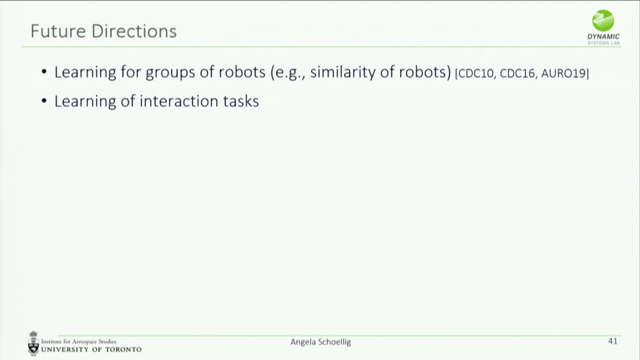 But I think you know there's many, many open questions, And some that I find interesting are: how can we, can groups of robots learn like? when can knowledge from one robot be transferred to another? What is the measure of similarity between robots? 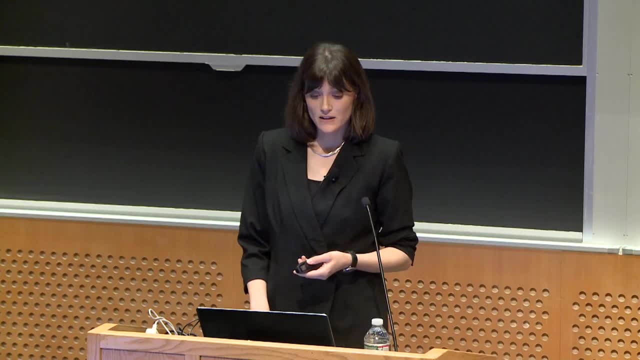 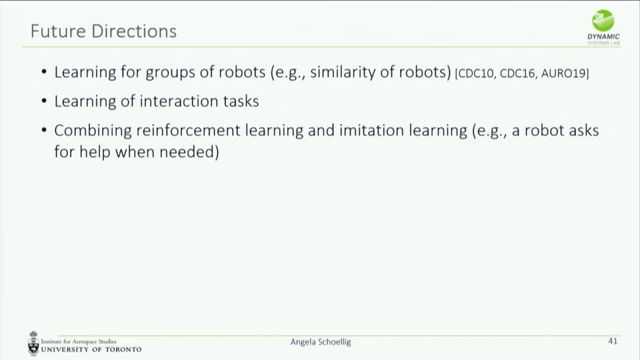 How can we extend these techniques to interaction tasks? Do robots actually interact with the environment? I think also an interesting question is: how can we combine reinforcement learning and imitation learning, So can a robot ask for help when it's needed and a human could provide input? 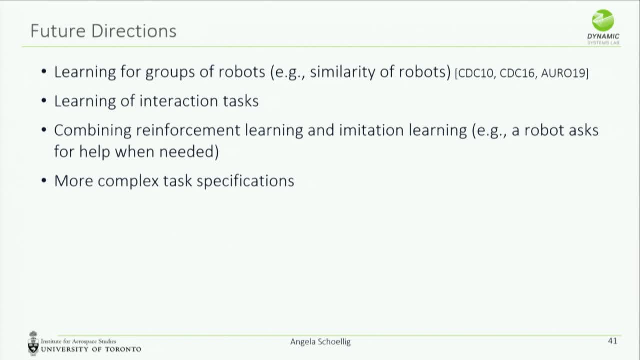 Then we got stuck with Stability and maybe trajectory tracking, but what about much more complex task specifications, Again, long-term and short-term learning and how to trade that off And how to eventually couple perception and control? Because really what we see in robotics is that almost every single module. 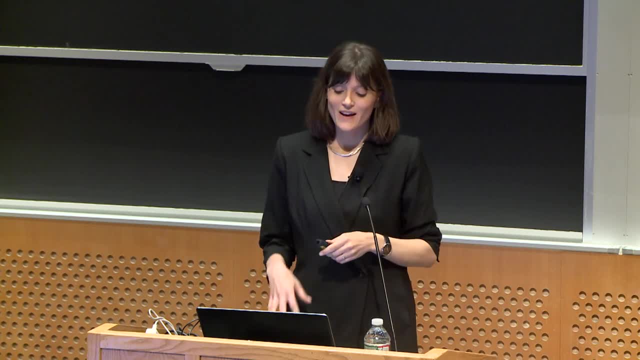 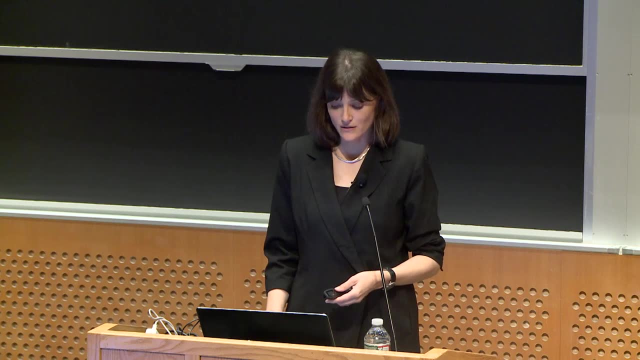 in this closed-loop system from perception to control, has learning components incorporated at this point, especially in applications? Okay, Thank you. So I think we're going to move on to the next slide. So we're going to move on to the next slide. So we're going to move on to the next slide. So how do we analyze and how do we design And how do we analyze the application areas like self-driving cars? So how do we analyze that and properly design that? 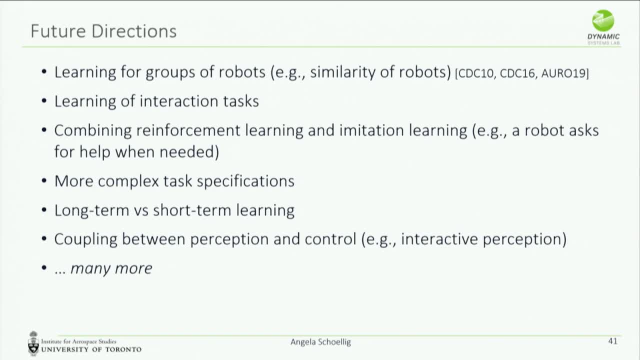 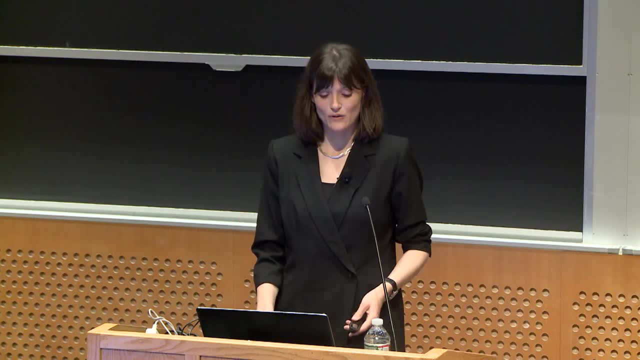 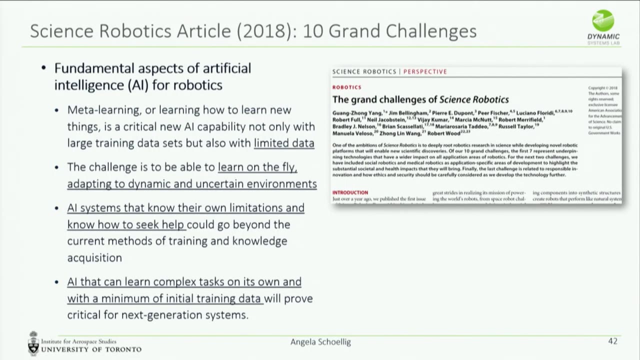 And so there are many, many more questions. I think it's an interesting area, But people have made progress in small ways, but I think there are many open questions. So if you are not convinced and think this is not true, read the Science Robotics article. 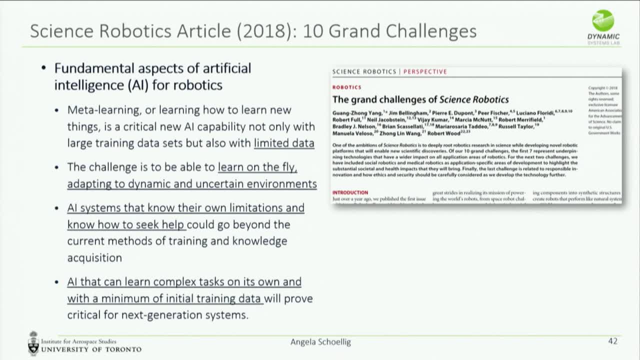 where they highlight 10 grand challenges in robotics, and one of them is aspects of artificial intelligence, and they highlight things like limited data, learning on the fly, enabling robots to seek for help and generally doing complex tasks. With that, I'd like to thank my team collaborators. 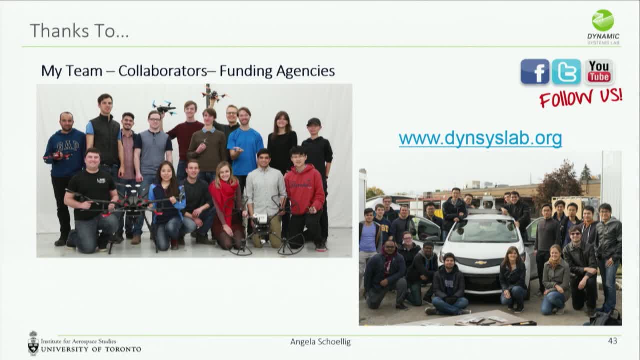 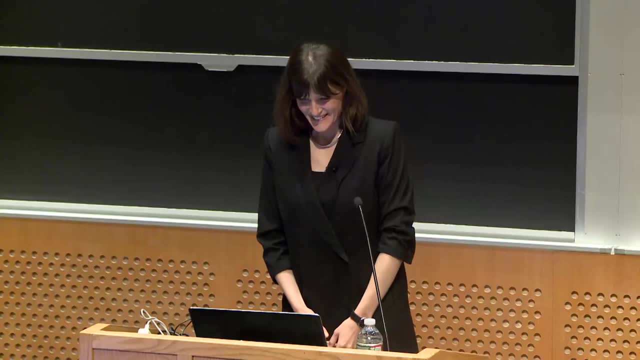 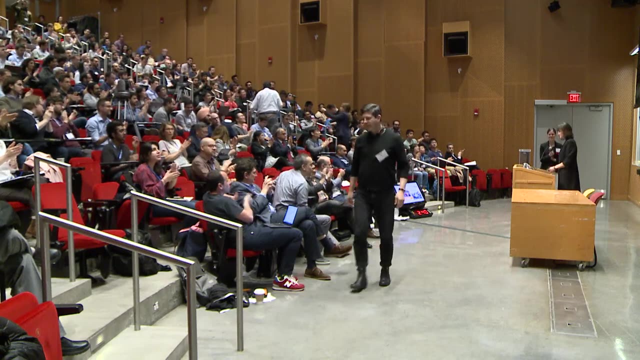 and all the funding sources, and I'm happy to discuss more of our work later, and if you are interested in joining my crew, please let me know. Thank you very much, Angela, for the very nice presentation. Everybody is keeping so well in time. 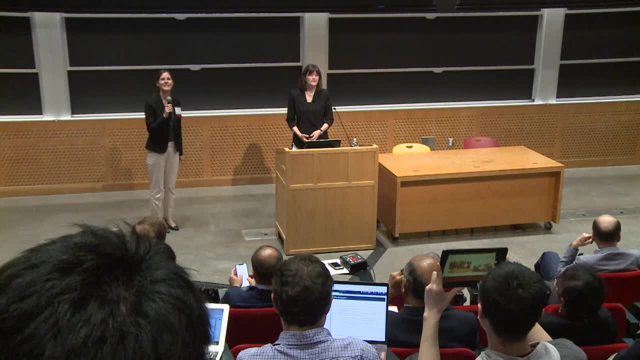 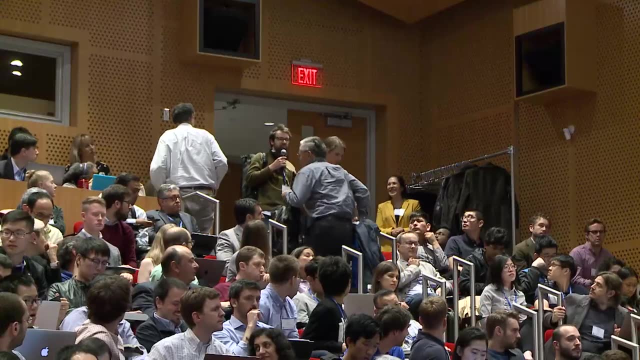 so we have enough time for questions. Yes, we start in the back. Yeah, Hi. So I really I think the idea of having the adaptive control in the inner loop is a really good idea. Just one sort of technical note about that L1 controller. 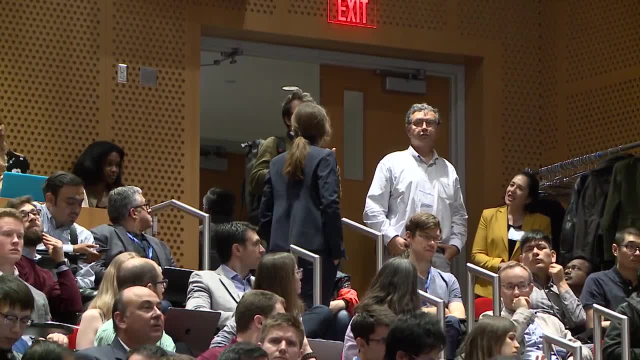 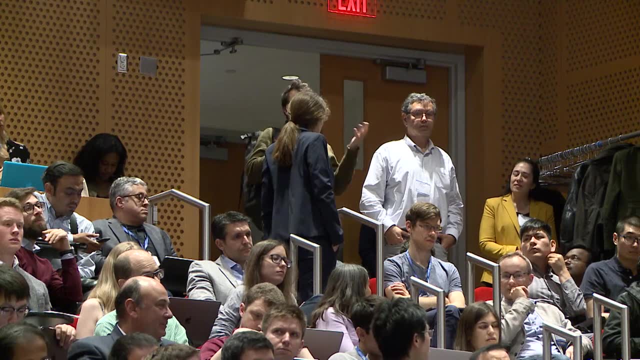 That bound of 1 over gamma isn't sort of unique to the L1. It's actually there's a fundamental, a general assumption in L1 that they have perfect matching and that bound actually isn't uniform. So that's just a feature of the assumption of L1.. 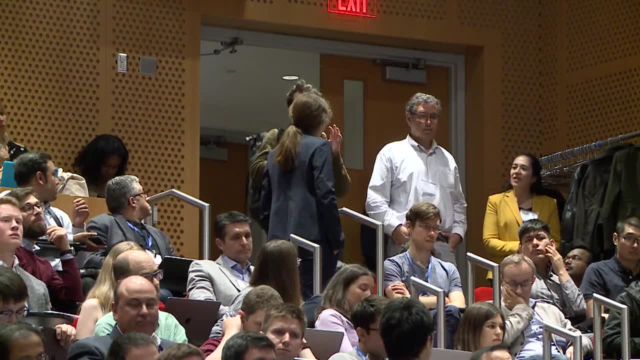 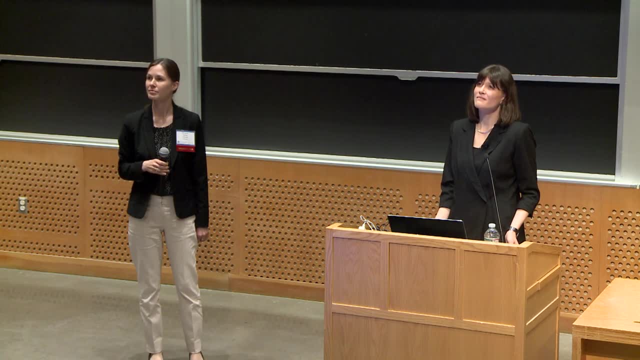 Yeah, So you should like just sort of caution, you that? yeah, So in the case of output feedback- actually, in the papers from that group, they initialized the reference model about state data, which they could never know. 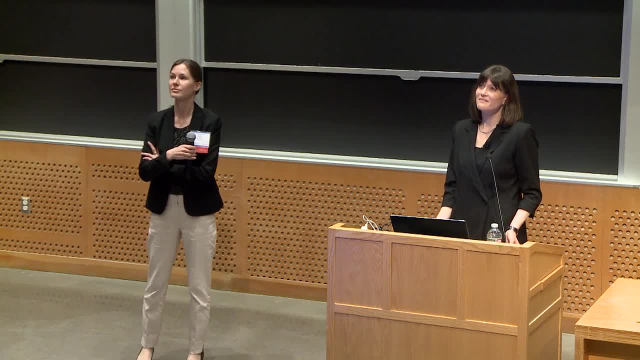 So that's just a generic feature that falls from the Lapna function and sort of the sum of squares of error, that. so it's just a general feature. just a general feature. So everyone knows It's not unique to L1.. 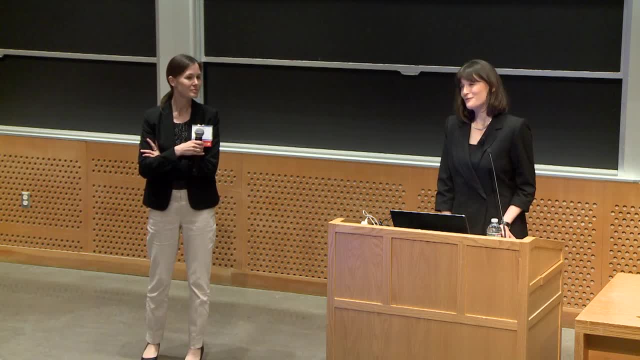 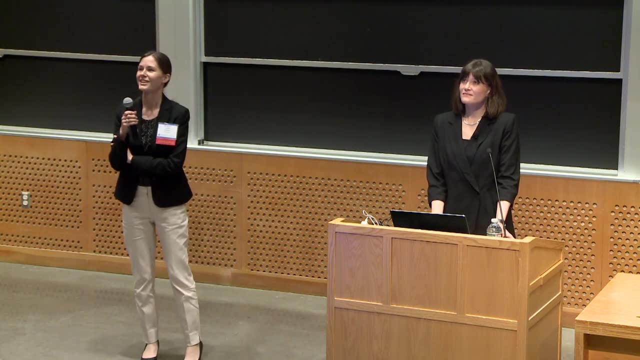 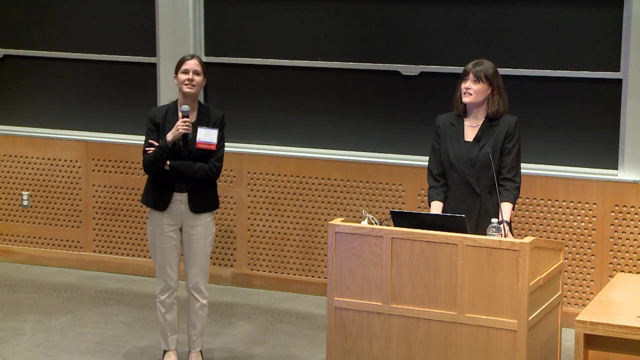 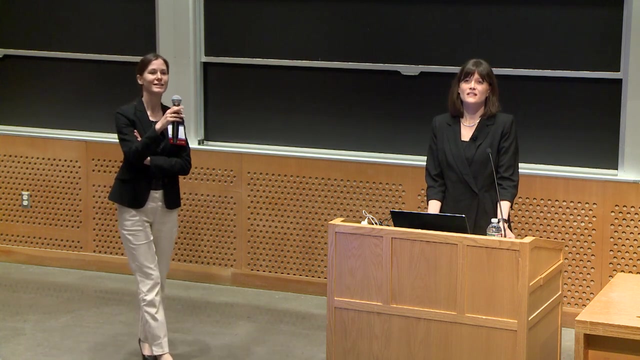 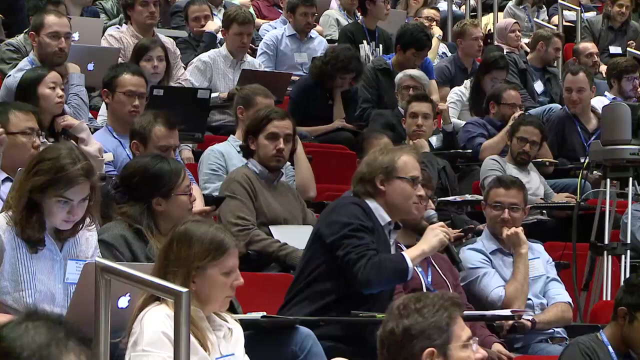 Yeah, I totally agree, And we are currently working through some proofs and had to redo a couple of them from the papers. Yeah, Excellent, More questions. Yes, Sebastian, Thank you, Okay. Yeah, So I have a question about the trajectory tracking. 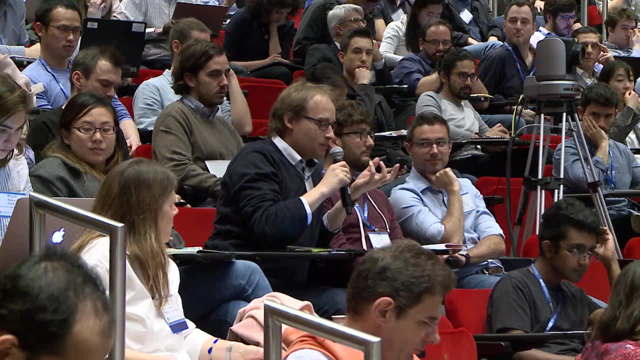 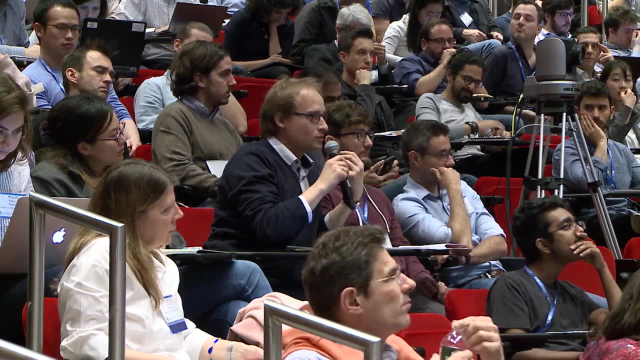 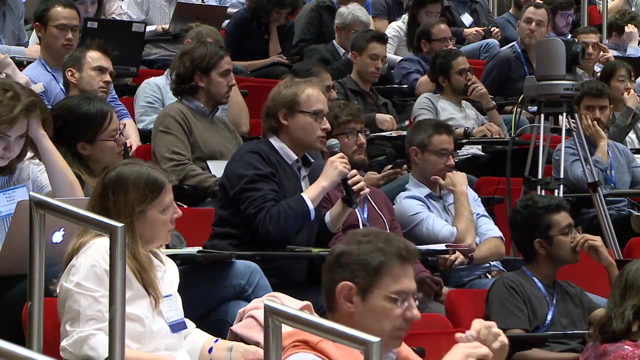 which looks very impressive. So do you retrain the neural network for every new trajectory And if yes, is there some hope that you could, if you've seen enough trajectories for these quadrotors, basically have a general neural network that you could use for all sorts of trajectories? 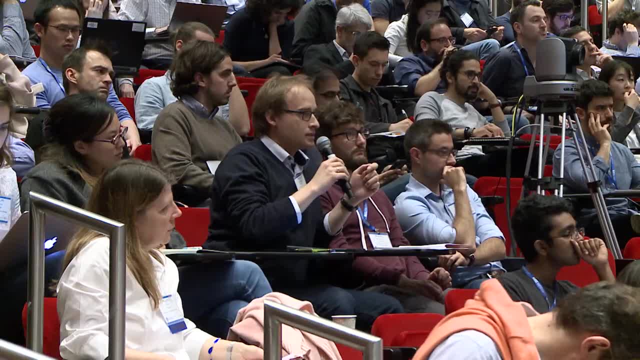 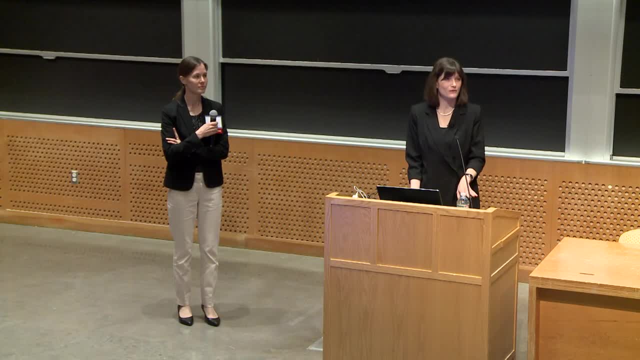 You're talking about the hand drawing, Exactly, Yes, Okay, Yeah, It's a single neural network. Yeah, It's a single neural network. Exactly Yeah, It's a single neural network network and it is trained on periodic motions. only the the results I show in. 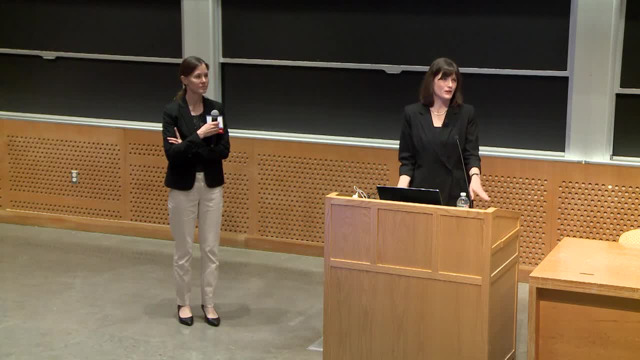 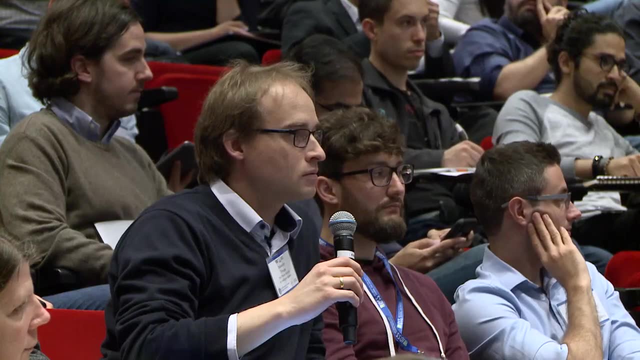 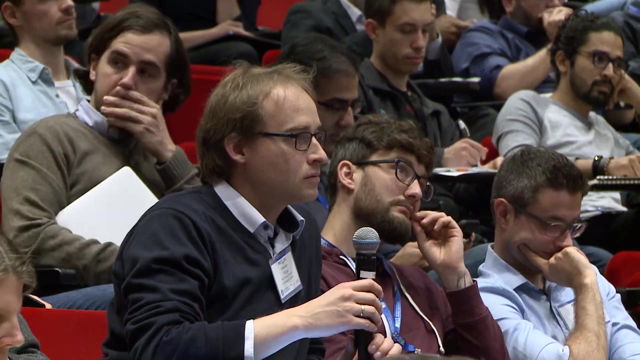 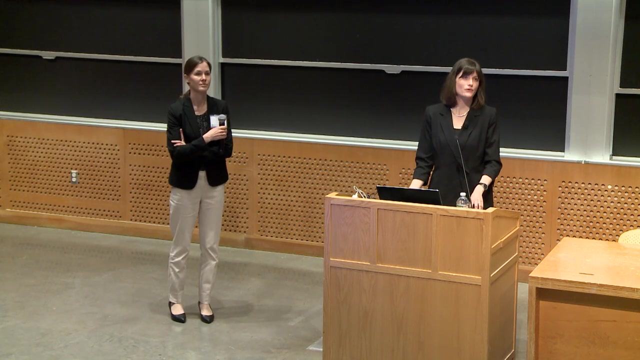 the showed in the video, is trained on various periodic motions with various frequencies, but not even on hand-drawn trajectories, and that's enough. and then we can show that actually, if this inverse would be unstable in the, in the, the ideal inverse would be unstable by the right choice of input features. we 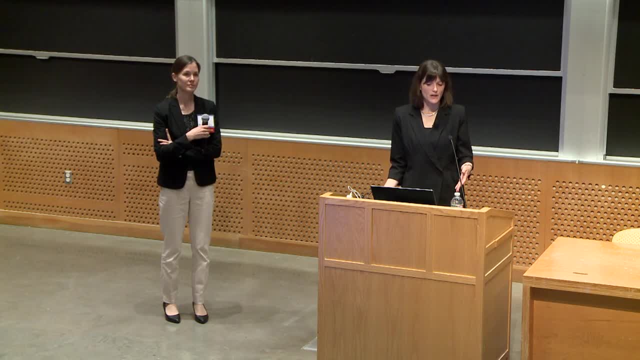 approximate the stable, the state of e. we learn the stable approximation and that is similar, in the simplified case, to some of the results that have been out there long before. okay, and do you know when? do you have an idea of, when you have enough data? no, that's a very good question and